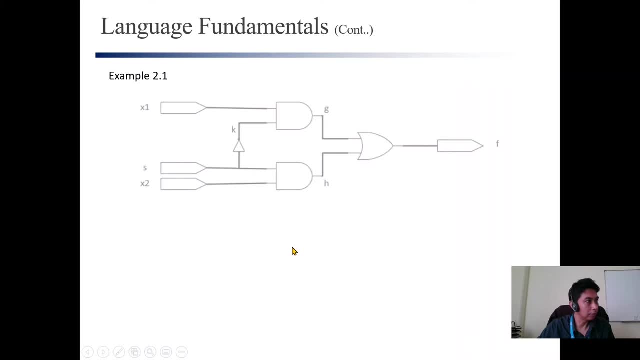 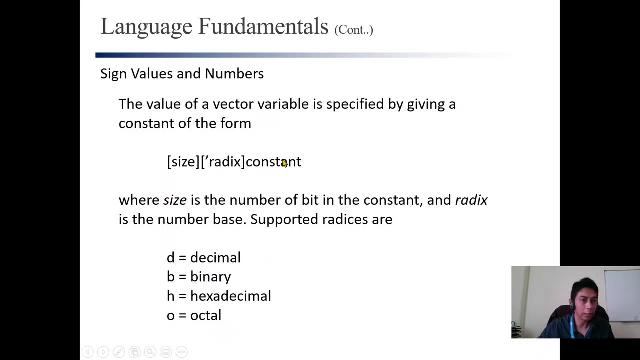 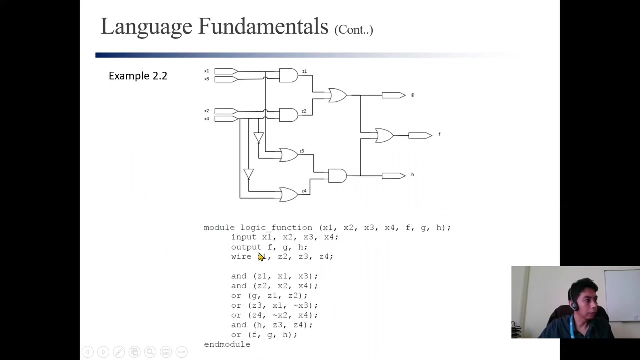 memorize what we call the definition or the terms or what. So this one is for your reference. So next time when you do the design, you start to code, so when you don't remember how to instantiate the gate, for example, so you can go back And this is what we will do. 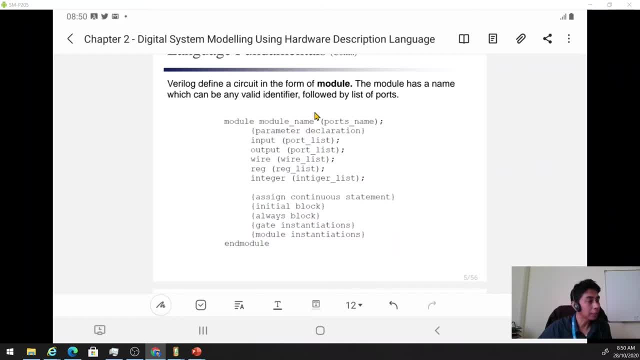 after this: yeah, the rest of the course. all right, so we will write the code for every, every circuit that that we have, that we want to design, right? so the general structure of the code is always like this, and you will start with module and your circuit name or module name. 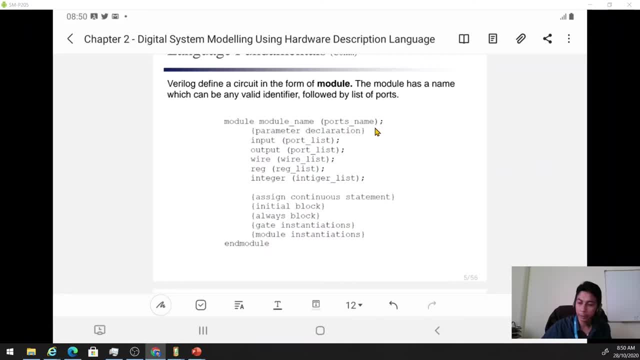 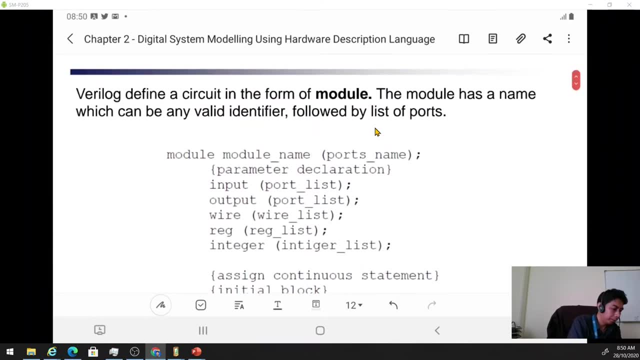 and the port list and the list of the port. so, for example, you have for design like this, then your name is will be a, b, c, f1, f2, right to the port of your design. so inside, here is your design and uh, you may have. uh, here is the. 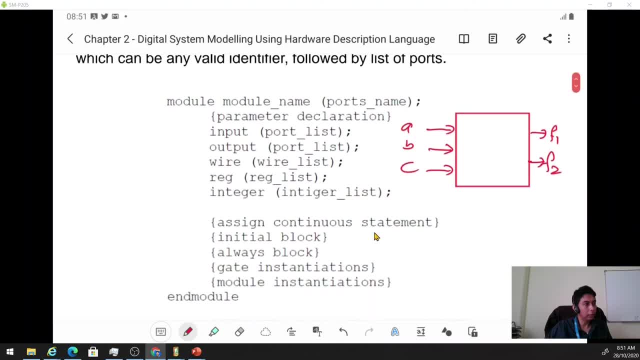 declaration part. all right, you need to tell the software, the quarter software, that, uh, which one is the input, which one is the output? so the output of this output list, input list, for example. so in this case it's a, b, c, output, f1, f2 and you. 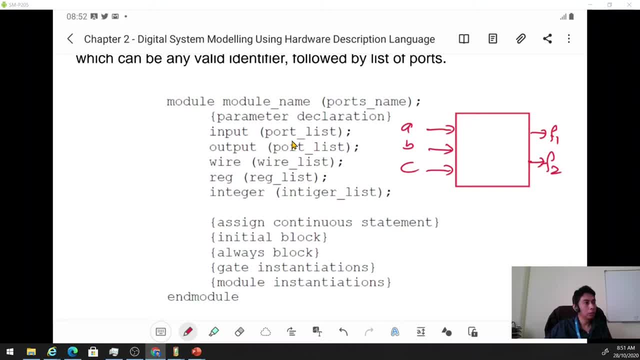 have. you have the option also, for example, a is one bit, in this case it's one bit. so if you have more than one bit, for example it is two bit or big eight bit, all right, so you have. you will have an option also to uh, to tell the software that the size of your, your input. 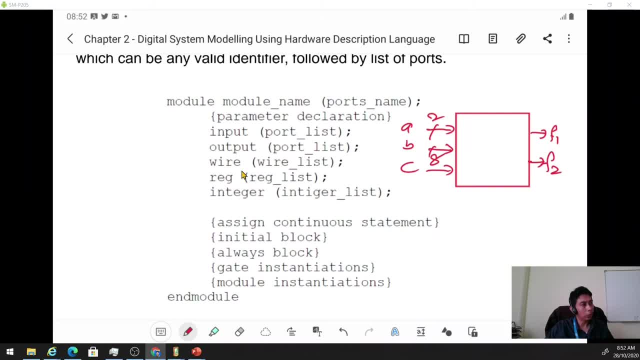 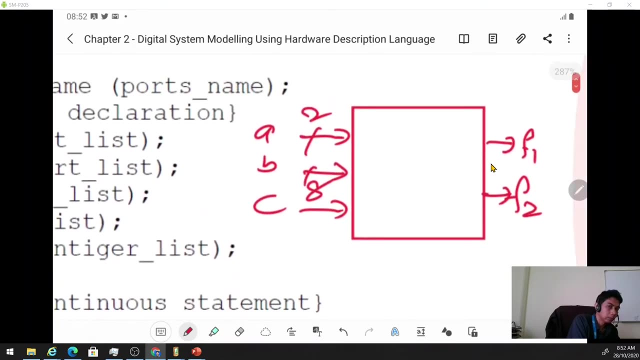 yeah, and you can have also: uh, why you like, what your declaration, what year is the connection inside your module? just okay. so, for example, you have sub-module here and sub-module here. this is connect to output and this one is maybe connect to the input and you have internet connection. 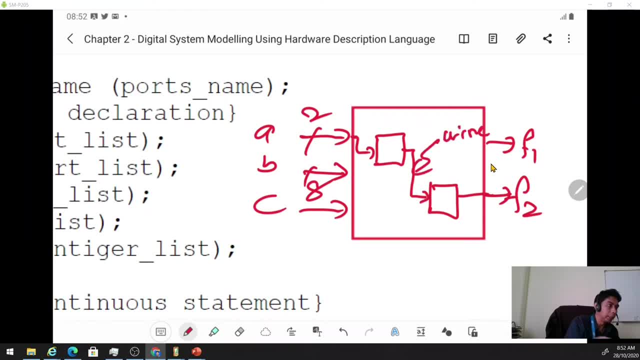 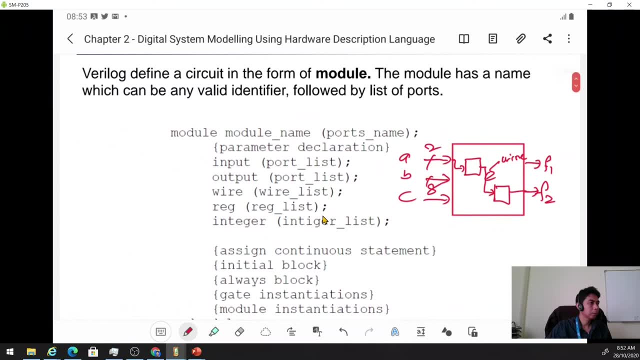 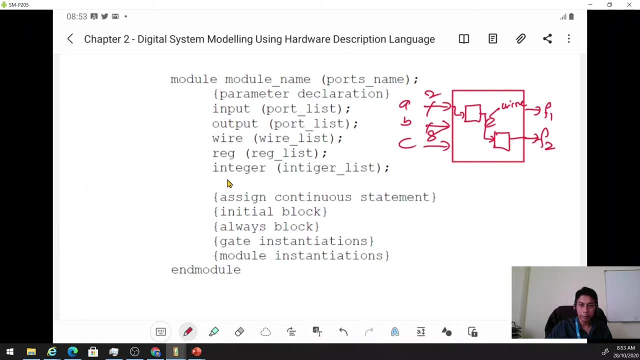 like this. so this will be uh for you, right, uh, right. and integer is the uh variable in very long. so sometimes in programming we always we will use the variable in in code, in our code. so later we will see what is right, what is integer and parameter declaration. sometimes we want to represent a number that we use many, many times. 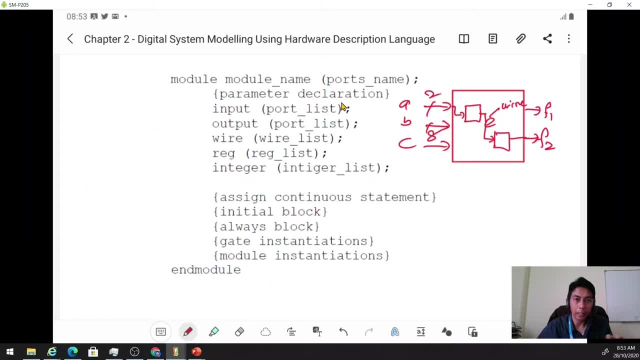 in our code. so we want to represent that number with a label, a name, so we can use our parameter declaration. all right, and this is the uh description, the description of your circuit or the body of the your, your code. yeah, so there are many, many ways to describe your circuit now. 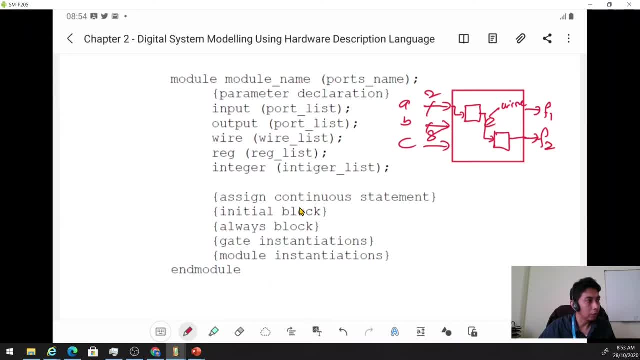 first one is we call us uh assigned continuous statement. so this one is the uh continuous assignment. we call it continuous assignment where uh, when you have many, many continuous assignments, right, for example, um, you have uh. so the assignment is simply uh, simply an equal symbol, and this is what we call assignment in very long. 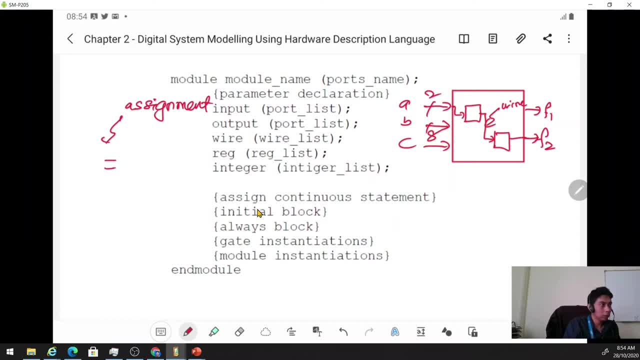 all right. so, uh, for example, you have boolean equations a and b, f1, f2, a or b and so on. so this, and, of course, in front of this, you need to use a time keyword, right, and this one also assign keyword. so when you use this, meaning that this statement, these two, 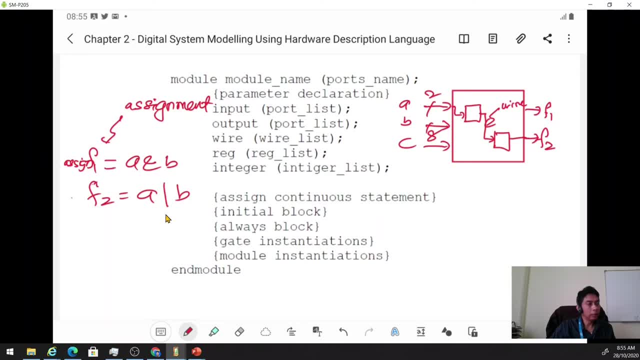 statements are running in parallel, executed in parallel, all right. that's that we call continuous statement, all right. so if you have more means that all of your this equation will be executed concurrently, all right, or at the same time, all right. that is a continuous assignment statement. the next one is initial block. 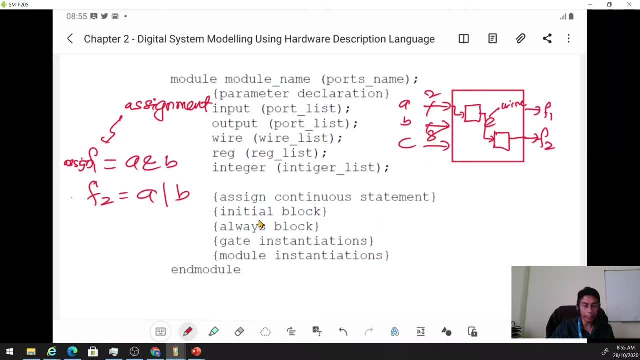 initial block is used when we do uh simulation later on. so i have actually created the video to use when we do simulation later on, uh. so i have actually created the video to not expect to show to you how to design using Quartus and to simulate your design. so I will share after the class so you can refer to the. 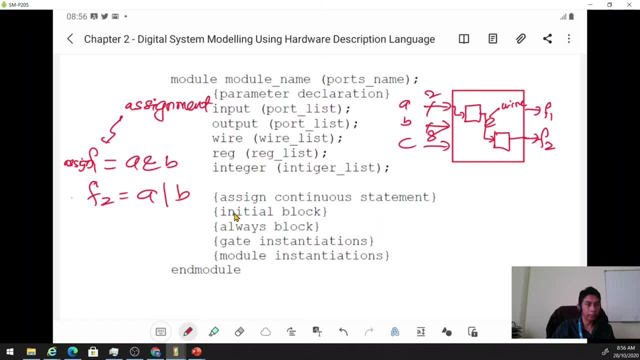 tutorial video to use Quartus and if we have time today also, I will show you how to how to design using Quartus. now, always block is when we want to describe our circuit using behavior, behavioral description, all right or sequential sequential statement. sequential assignment statement. sequential statement. 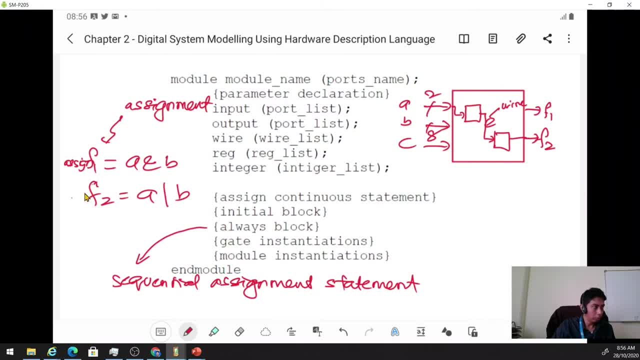 all right. so if you, you have your bullet equation inside always, law even be, it will not be executed in at the same time, but it will be executed in sequence. I mean that this one first and so this one, and so on. that's why we call sequential assignment statement. yeah, right, gate instantiation is what is. 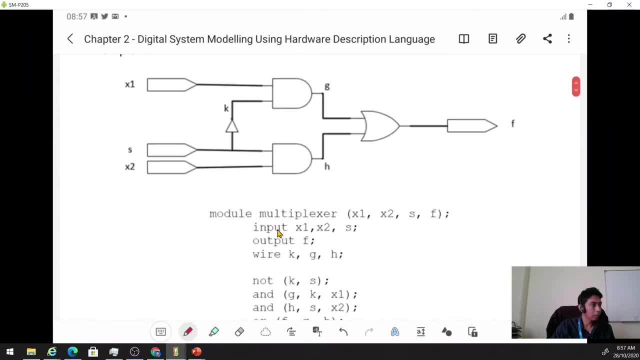 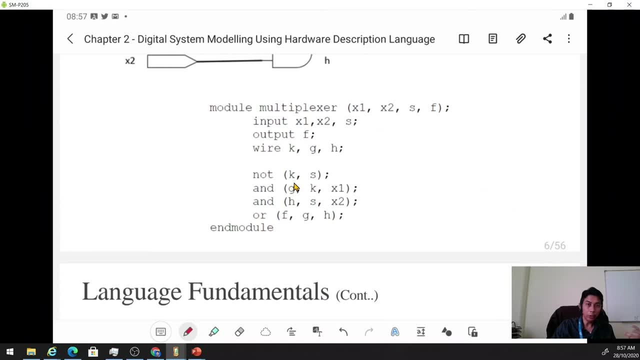 getting a sensation when you do this. this is gate instantiation. mean that you, in your code, you instantiate the gate. so in your code you see it very clearly. oh, this is not it. you put on, get there, you put and, get there, you put in. this is called gate instantiation. 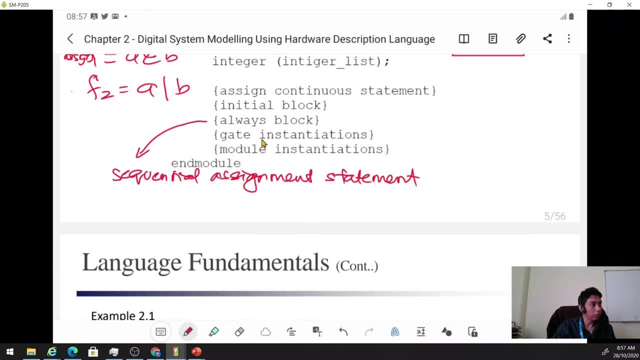 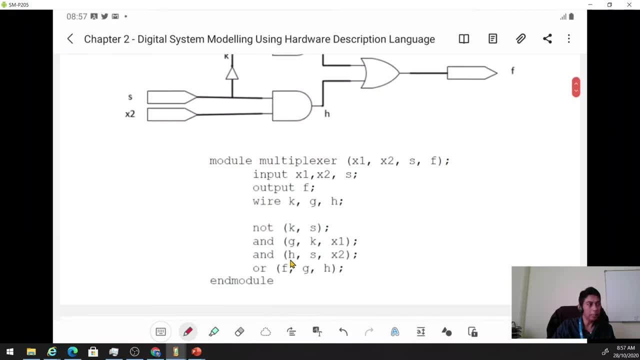 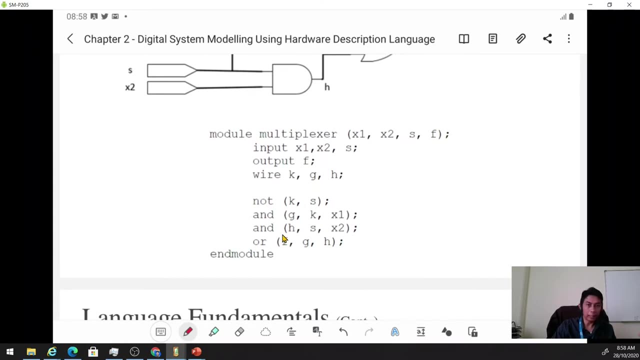 um, now what we have, module instantiation. module instantiation is uh is similar to get instantiation, but instead of we instantiate the gate here. gate here is the standard library means that means that we use the internet library of of the software, but module instantiation means that we use our own. 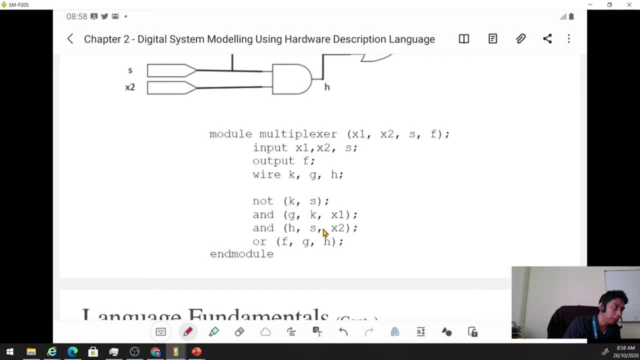 circuit and to instantiate our circuit, for example, you have your design, all right, the design, the big design here and inside your design you want to use, reuse your previous design. right, this is your previous design, for example, under the previous design or sub module, all right. so when you 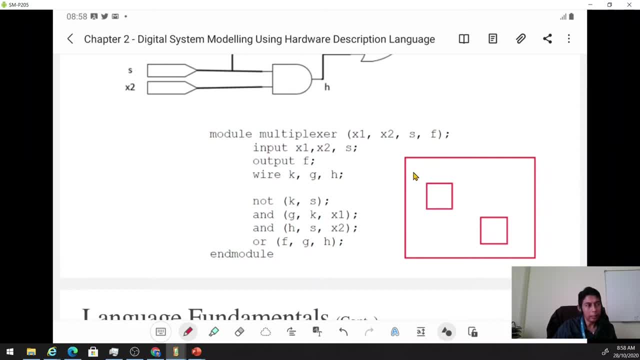 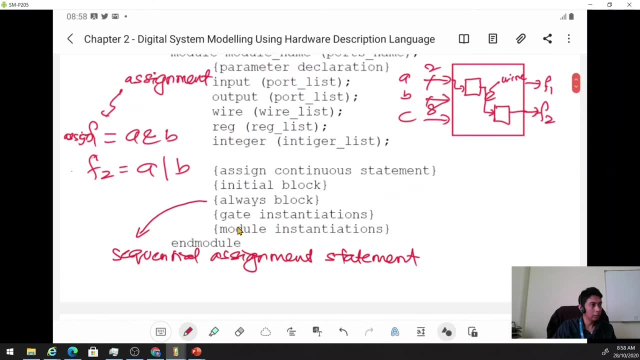 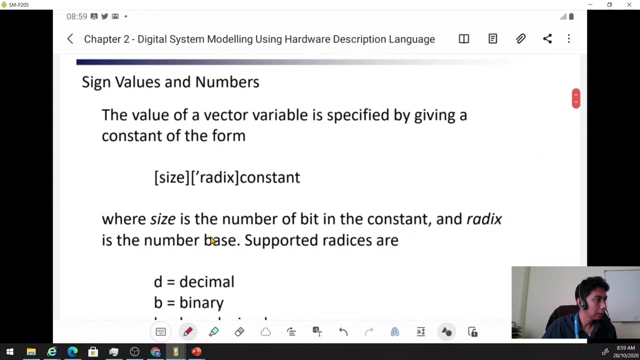 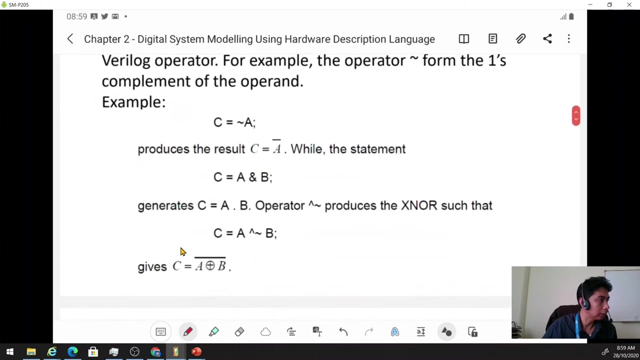 instantiate a module, all right in your design. okay, that is called module instantiation. okay, so there will be a uh, a lot of ways or methods in uh, in describing the circuit in very long, all right. so you see, i think number is done right, parameter, everything. so i explained already so i will keep and go to the 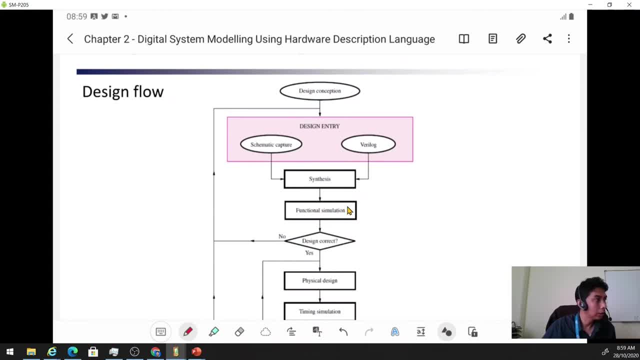 here, right where we stopped last week, all right. so this is uh what we call the design flow, where, which is the step right that you, all of you will uh go through when you design your circuit in this course, all right. and, of course, for any design later on, when you want to design, for example, you do. 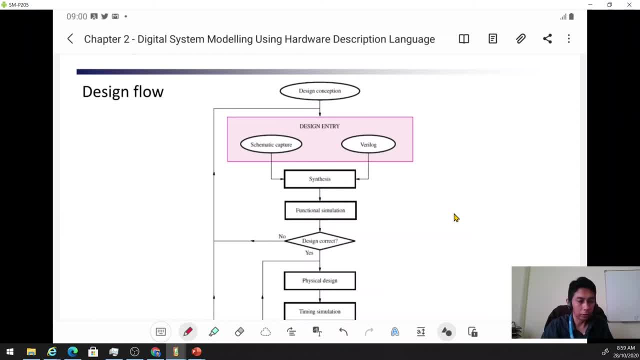 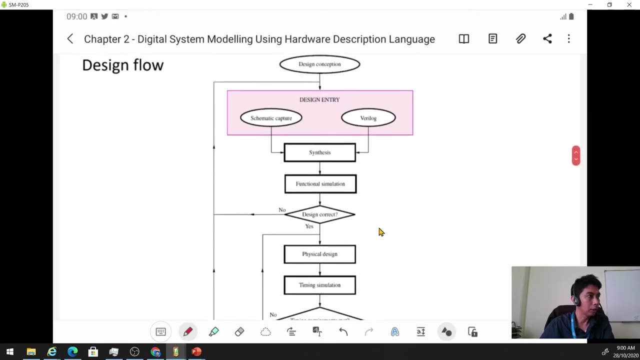 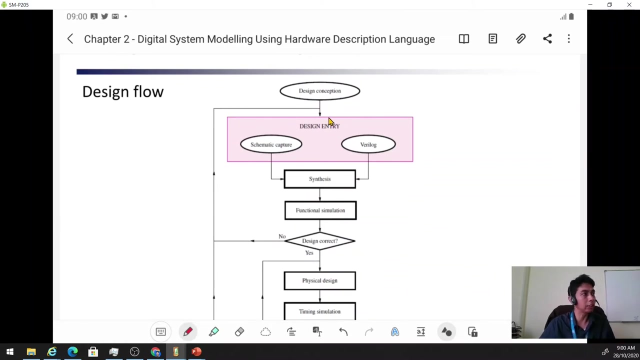 the project, or after you graduate, in your work, when you become a design engineer. so you use this design flow to design your circuit. all right, so what is the? what is inside? what is the process? so the process will be this: you will start with design, description or conception. so, of course, 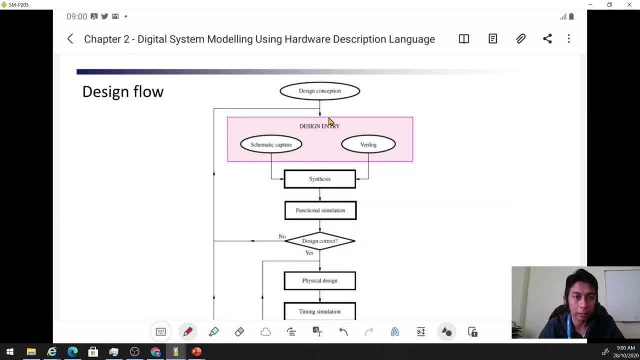 if you want to design something, you need to have the specification right. specification means that, for example, you want to design a traffic light controller right, so you need to know how many junctions you have right, how many traffic lights, how many lights you need, and what is the sequence and what is the timing. and so 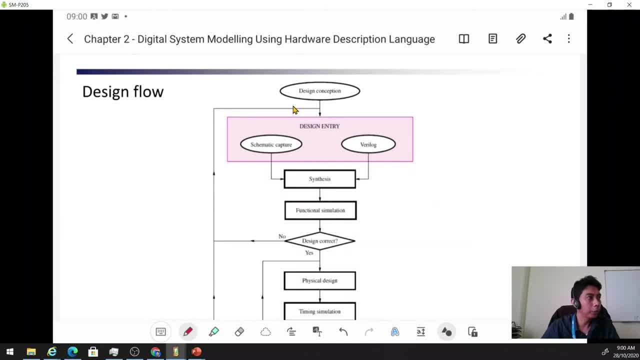 on. that is called specification. all right. so from specification then you start to design. all right. so normally we have two type of design entry. we call it design entry, design entry. first one is using schematic. all right, so I think if you learn digital electronic you will design using schematic, capture a lot and using 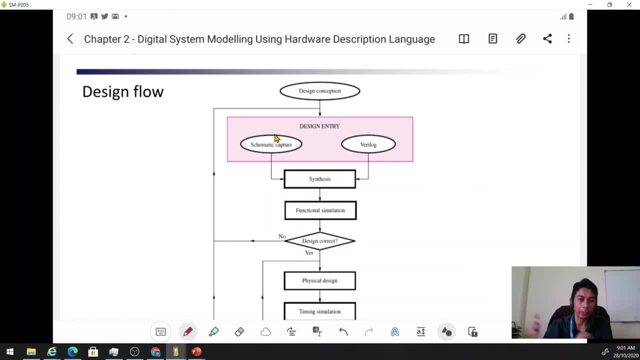 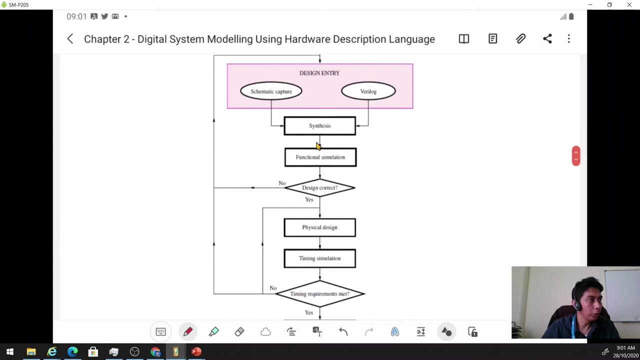 schematic means that when you draw your logic gate and connect to gate or connect to this gate and this gate, so that is schematic capture, all right, but in this course we've been used very long language to describe our circuit. instead of schematic capture, schematic, all right. and after you have your code now done, what you need to do is: 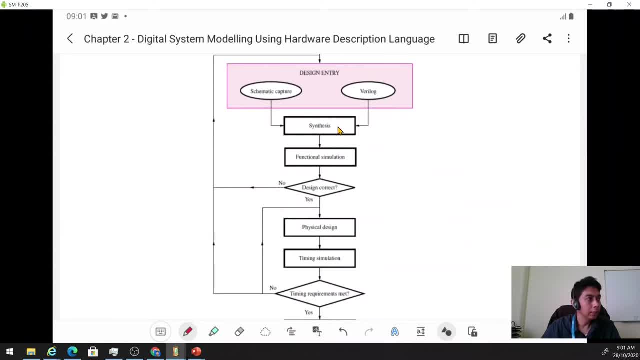 synthesis now, what is it? synthesis is the process of onwarding. onwarding the language and your, your program, your code, now into the net list or into the schematic. all right, into the net list now means that if you say this gate is connected to this gate, then you are done with the code. 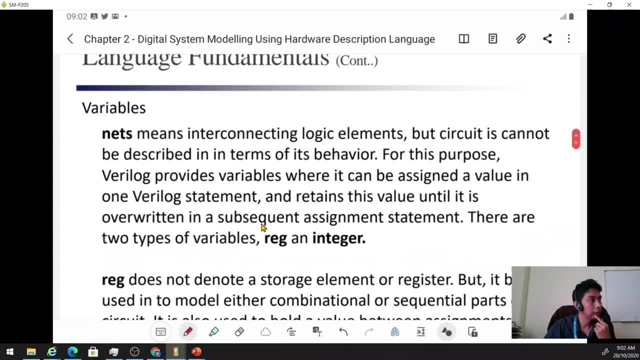 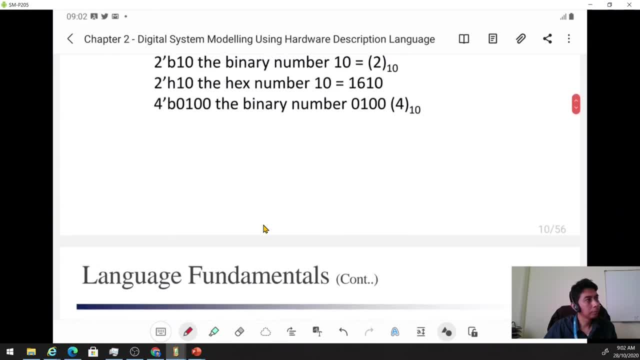 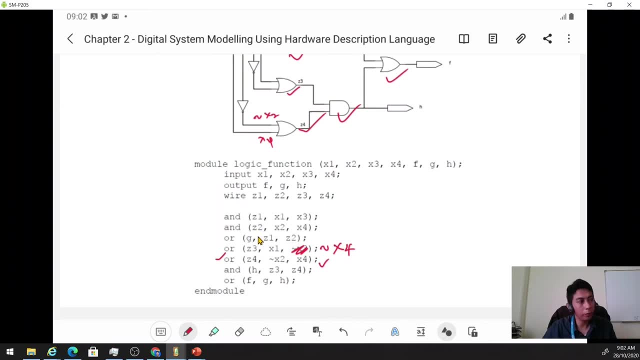 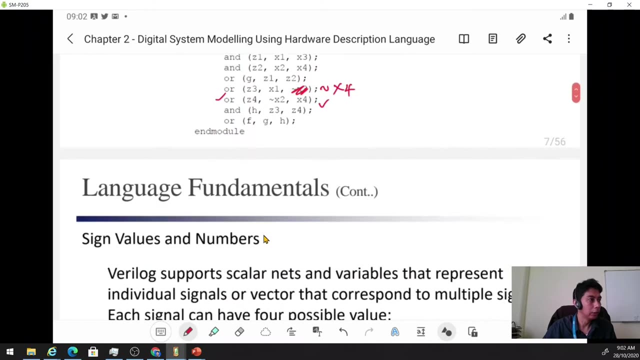 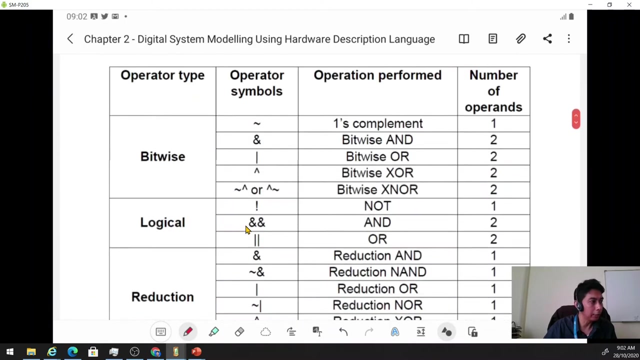 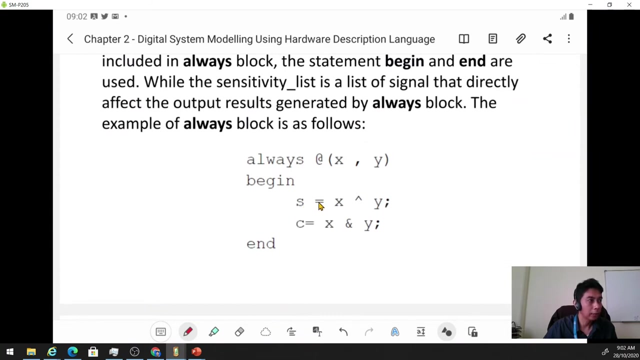 like this. this did connect to this kid, so the the software will, will try to, to synthesize or to create the circuit for you. all right, and this is good, because sometimes we, we, we design our circuit or we code our circuit using a equation like this right. so, for example, if s uh equal to x, this one is x or y. 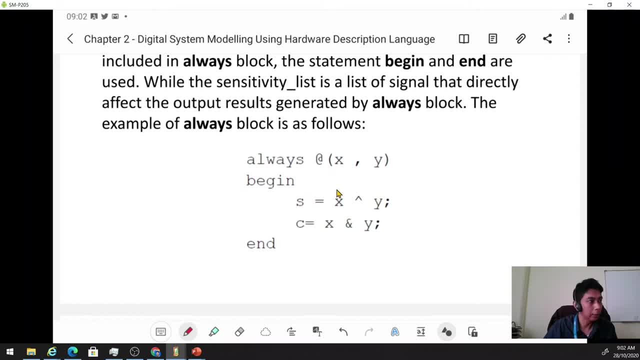 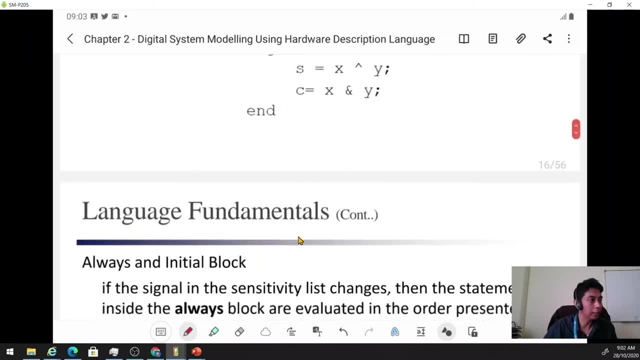 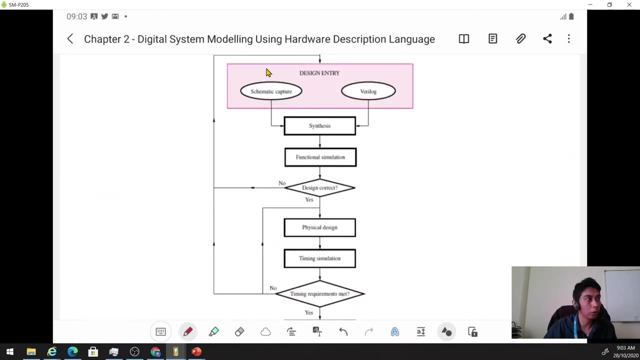 so when the software get this equation, it will produce the x of it for you, and the input is x and y and the output is s. all right, that's is called synthesis, and synthesis is done by software. all right, so your work is actually inside this, inside this. 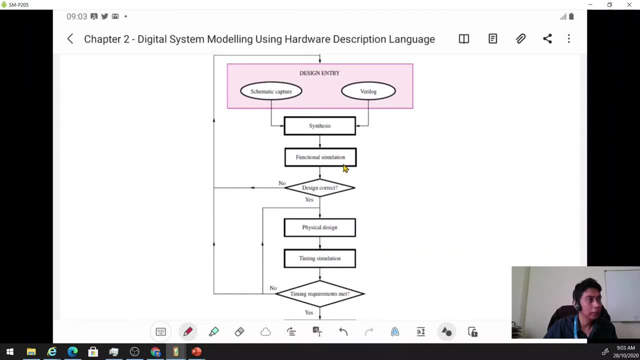 box. so synthesis is done by software and after synthesis if there is no syntax error and connection error. so connection error we can see in the. sometimes it will be given in warning, in your, in your purpose, and we will do what we call a functional simulation. so functional simulation is the first step of Destiny simulation, where you 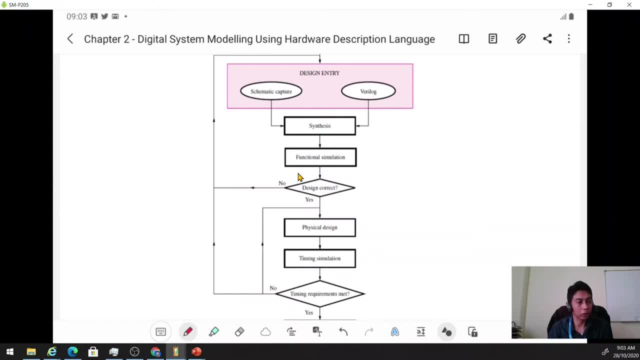 want to see whether the output is correct or not now, based on the input. so if, for example, when you design something you need, you should be you, you should know already what is the output. right, if i give this input, the output should be like this: all right, so you can use this to do the promotion. 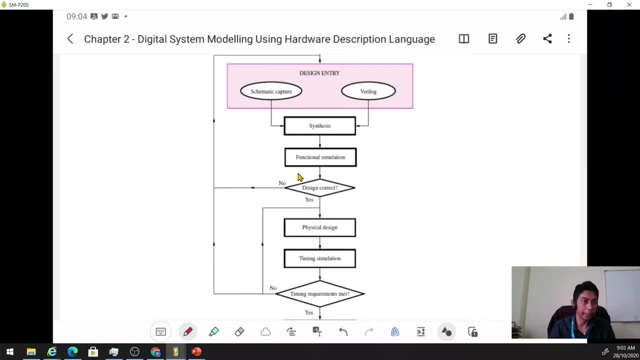 output: right? yes, so you can simulate your, your design, by giving the a set of input- all right, a set of input- and observe the output. if the output is not as expected, so means that your design is wrong somewhere, right? so if it is not correct, so you need to go back and look at your design again. 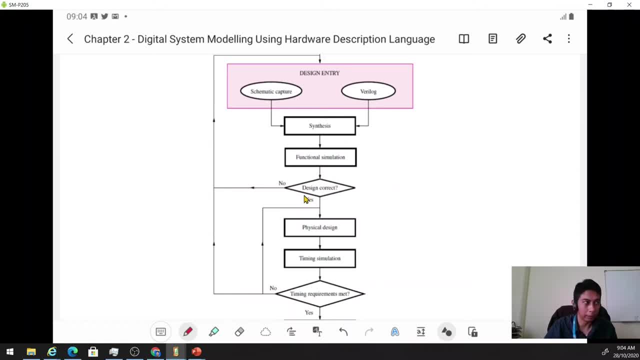 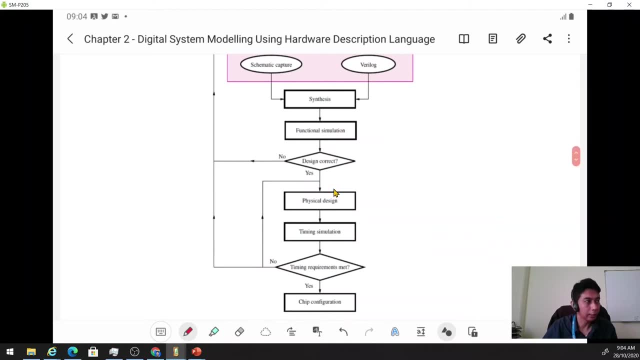 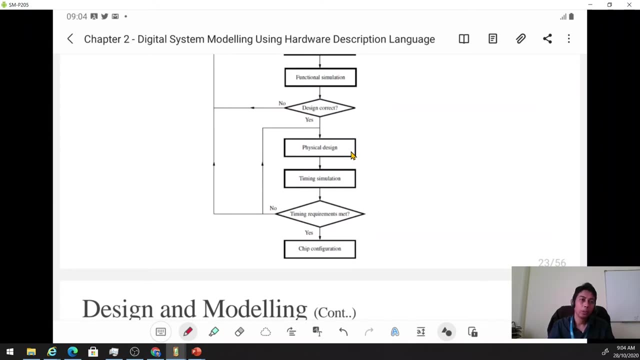 and do the synthesis and simulate again until you have passed the functional simulation. after you pass the functional simulation, your job is not done yet. all right, then you want to do the physical design. physical design means that you want to implement to the real hardware. all right, to the hardware and, uh, the hardware that we use. 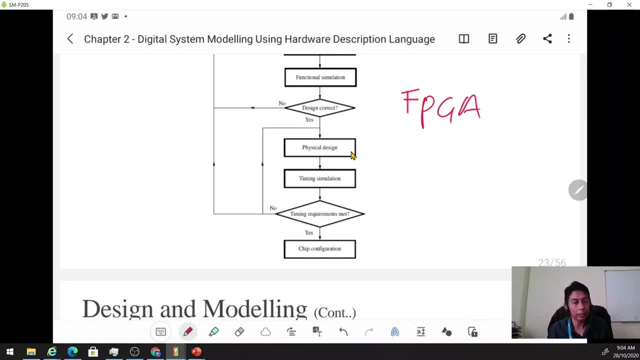 it's really, yeah, feel, programmable gate array. it's very popular nowadays, right, and this fpga in in the market. there are many, many, many versions. there are many, many types of fpga, so some is designed for low power, some is designed for high speed. all right, so you need to to have the right one for your, for your uh, for your design. so 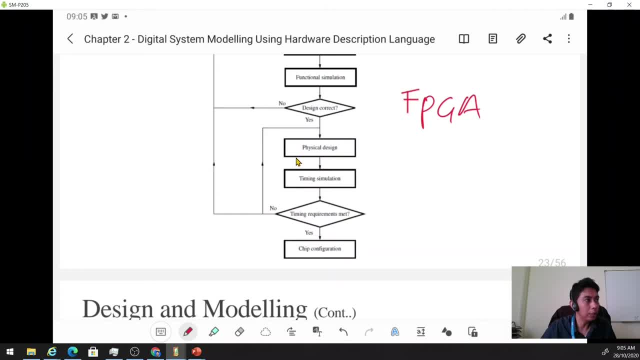 uh. here you need to choose uh, which is the device, your target device. you target for what device device? so in the software there will be uh when you install the device. last time, during the installation, you are required to select your, your device, family, right? so i asked you to to download the cyclone 2 until cycle 4, cycle 2 for cyclone family. 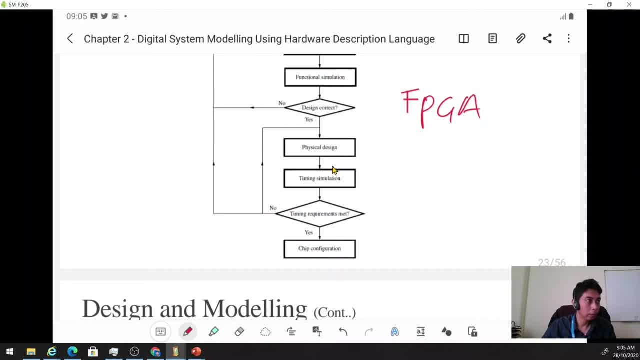 so, uh, when you use that one, we need to do what we call timing simulation, all right. so here you need to make sure that your design pass the timing right. for example, if your target is slow, all right, if your target device is slow, then you will. uh, you simulate, all right, you give. 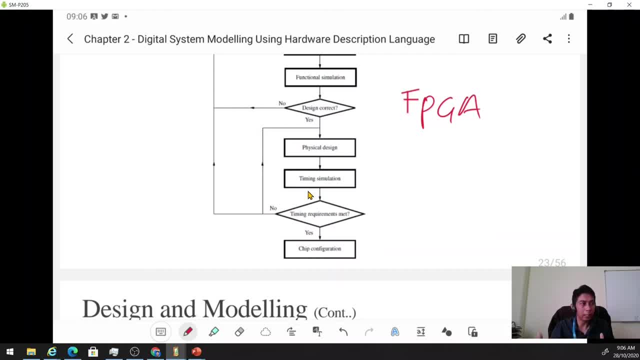 the input, the series of input, the is very fast, then it may not pass the simulation. all right. so if not fast, you need to go back and check whether your simulation is correct or not, or your design is correct or not. is it possible to implement in the low, low speed device or, if you want, to implement, in high speed device? so 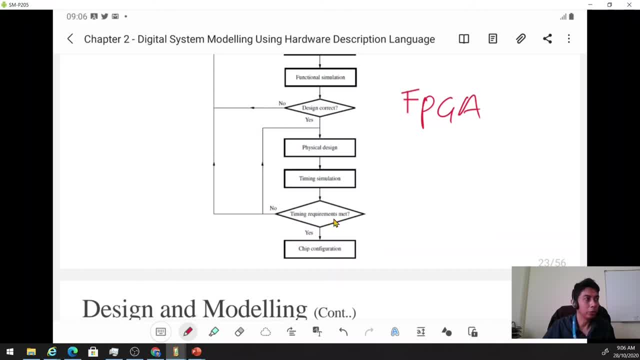 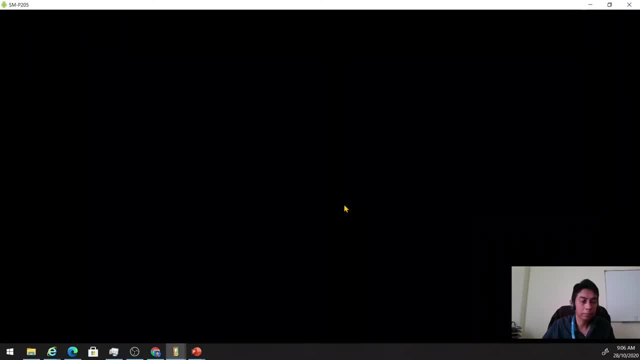 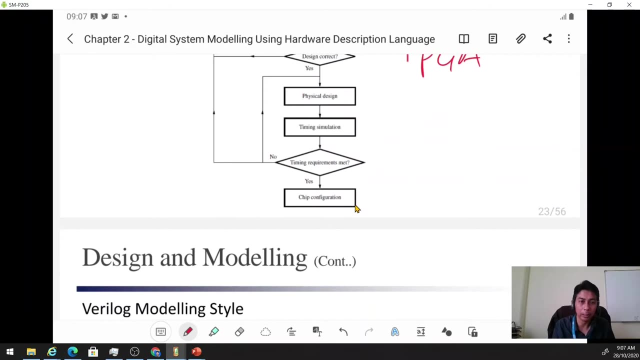 what is the design trick or optimization that you need to do? so that is called a physical designer. all right, so when the timing simulation is passed, then your design should be- should be ready for, for what we call cheap configuration means that you download. you download your design. 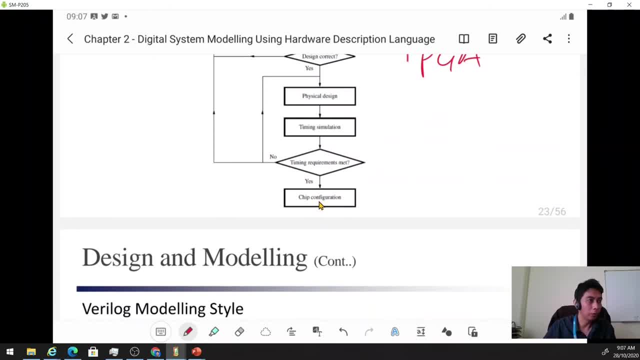 into the, into the chip. all right, this we call chip configuration of chip programming. all right, okay, so that is the design flow that you will go through this semester and we will do. we will not do the last part, the cheap configuration, because this one is the hardware and because 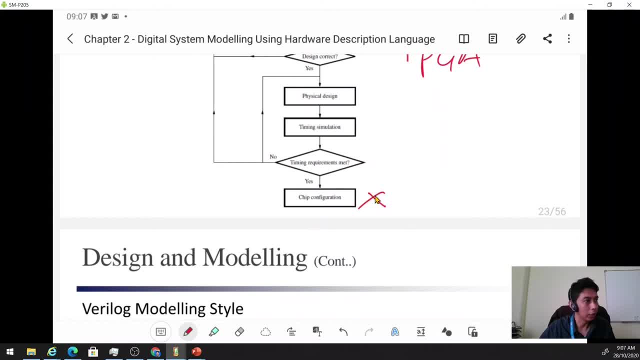 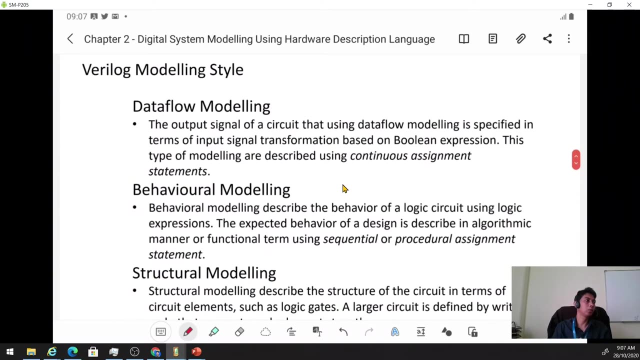 we, we are learning online, so we don't have we not be able to access the hardware. yeah, all right. now come to the very long modeling style in detail. all right, so what is modeling? modeling is, uh, how you want to represent your circuit. that is modeling just like, uh, you, uh. 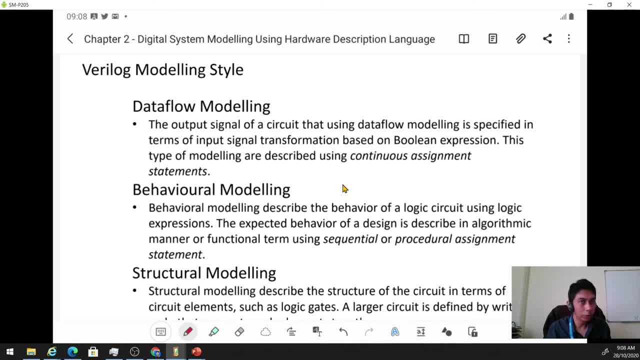 if you learn physics right when you want to explain atom. for example, when you draw atom with uh nucleus and photon inside at the center of the atom and uh orbit by the electron, that we call model. we call model, all right. so now it's the same. now we use language to. 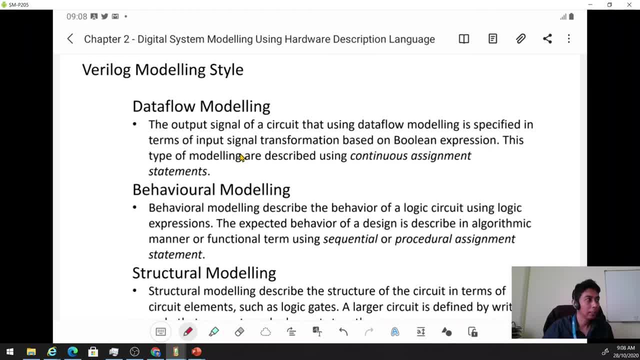 model, or to uh to represent the circuit. all right, so there will be three kind of uh modeling modeling. so first, the first one is data flow modeling. all right, so what is data flow modeling? data flow modeling is when you describe your circuit using boolean equation and use the continuous assignment. all right, so remember, if you use 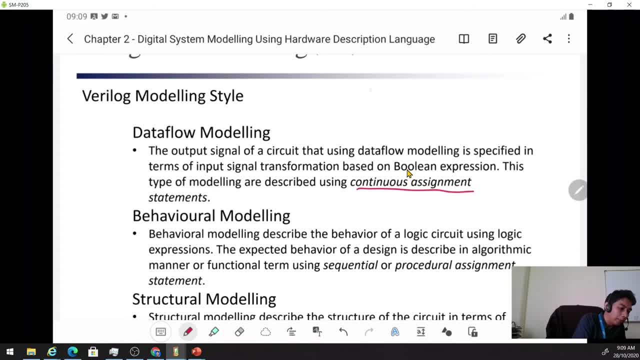 a continuous assignment. you get, for example, you have a boolean equation: f equal to a or b. right and in very long you write like this: assign f equal to a or this is all. yeah, this is all. and b okay. so this we call data flow modeling. all right, 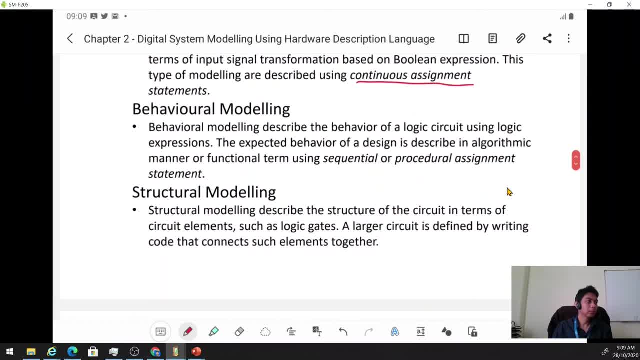 next. now, if you uh, design your circuit using uh or describe your circuit based on behavior of the circuit, that is called behavioral modeling. all right, and behavioral modeling. we will use the sequential assignment statement, or what sometimes we call procedure assignment, safety, sequential assignment statement. that is more behavioral modeling. 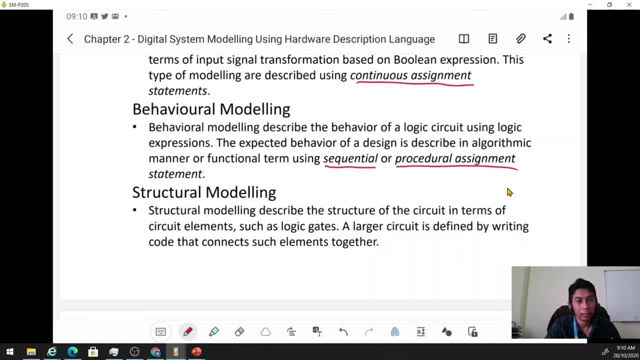 all right, so the same circuit you can design actually using uh data flow modeling and also using behavioral modeling. and the last one is structural modeling. structural modeling is when you instantiate the gate using the netlist or connection and, just like we we saw just now, when you instantiate the gate or when you instantiate the, the module, that is structural. 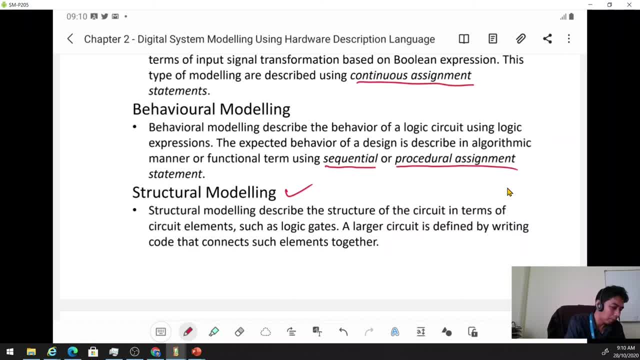 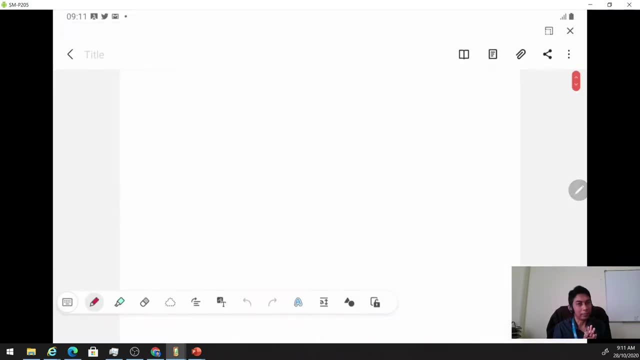 modeling. all right, so i give you an example to differentiate between the two, uh, the three, all right. so, uh, let's see the example here. so i give you an example, uh, how to differentiate between the three, and this is very important that you can help me, and if you understand this, i think my objective today is the same. um, okay, 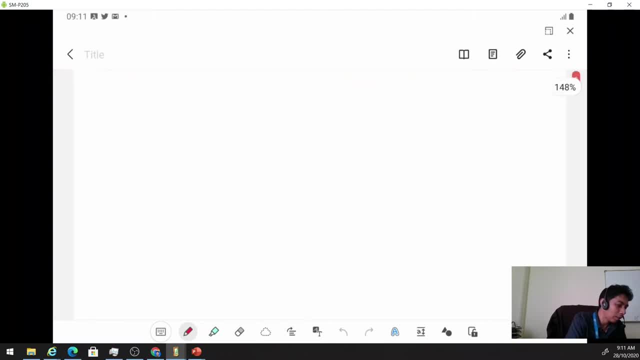 so, uh, first, uh. for example, we want to design, uh, i think the circuit. okay, so, uh, first, uh. for example, we want to design, uh, i think the circuit. this is the multi-flexor, you know multi-flexor, right, so multi-flexor, this is x1, this is 0, this is. 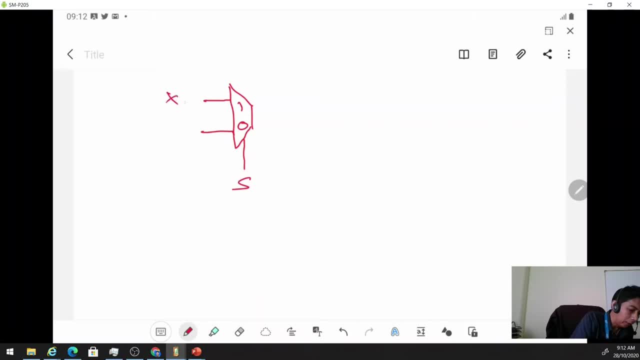 this is yes, select. this is x1, one zero and this is multiple, two to one, multiple uh. so what is the uh boolean discussion for? Yeah, so well, okay, we have x1 and you have, because you have how many inputs? you have 3 inputs, right? so the number of inputs? 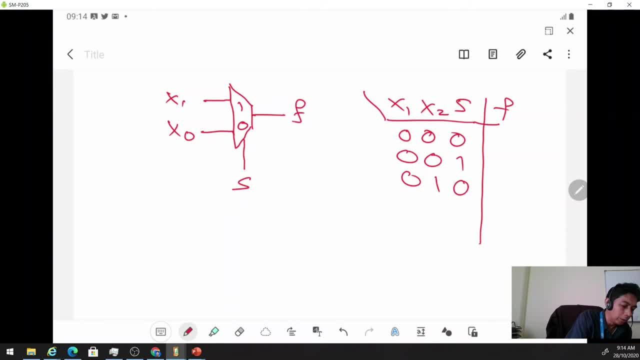 is called from: 000, 001, 010, 011, 100, 101, 101110, 1111, no and uh. you can calculate arrangement like this. i don't know what happens like this. i changed it a little bit. speed F here: x1, x2, because if F equal to 0, the output should be equal to x0, x0, 1, 0, 1. 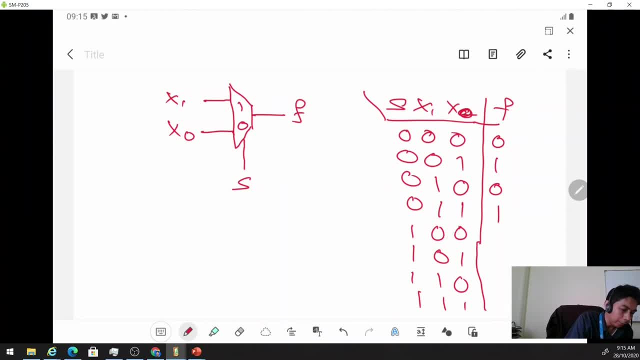 if F equal to 1,, so the output should be equal to x1,, it should be 0, 0, 1, 1, 1, 0, 0. so this is the truth table of the multiplexer and from this you can derive the Boolean equation which is F equal to. 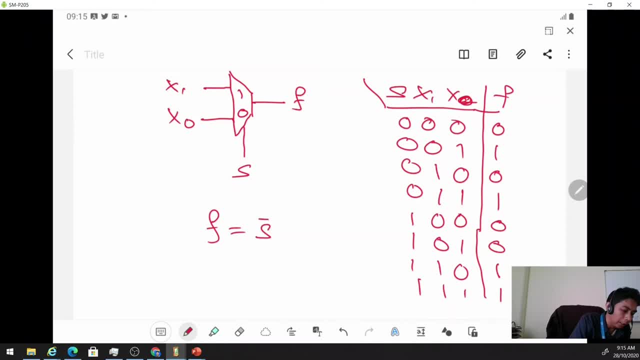 F as far as 0 or F as 1, F as far as 0 or F as 1, F as far as 0 or F as 1, and from this you can have your, you can have your circuit right, so your circuit, so you can have something like this: 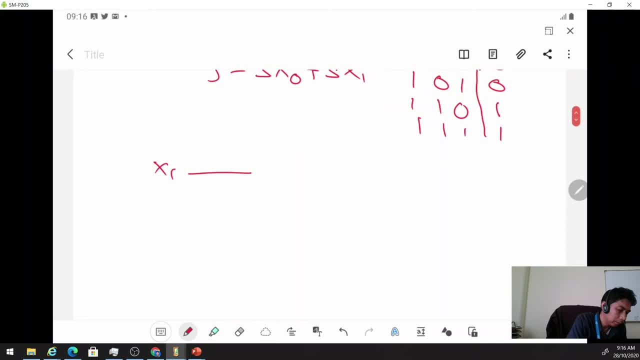 x1, x0, x1, x0, x1, x0, x0, x0, x0, x0, x0, x0, x1, x1, x1, n, and then you have cell for bit n like that, right? so this is the schematic for the multiplexer now. 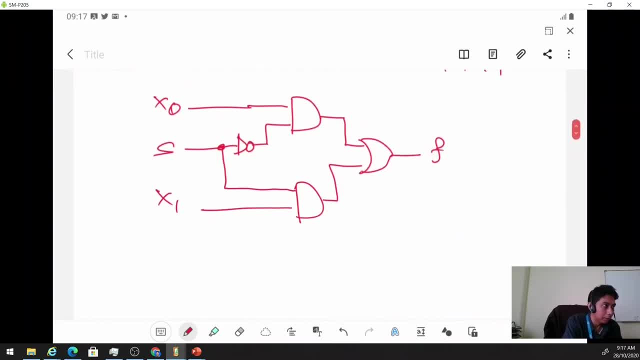 how to code or write the code for this one right? um, so we have three options. first, we use data flow modeling. all right. so how to use data from modeling? very easy because we have the equation and confirm multiply data flow modeling. right because first time when you want to use data for modeling, you need to have the equation. 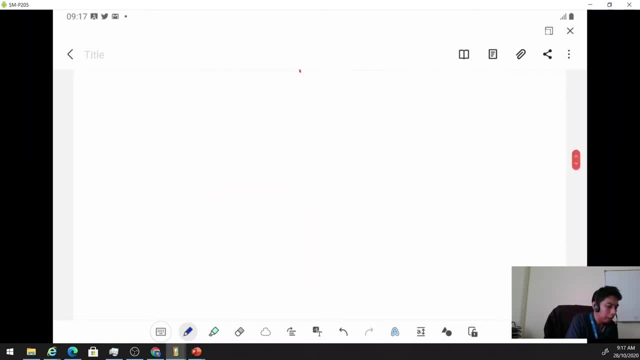 okay, so first you want to write the code. you need to start with module, then your module name. for example, we call it max. let me name. and what are the port, please? and what means a double? so you have f, x, 0, x, 1, n and x. 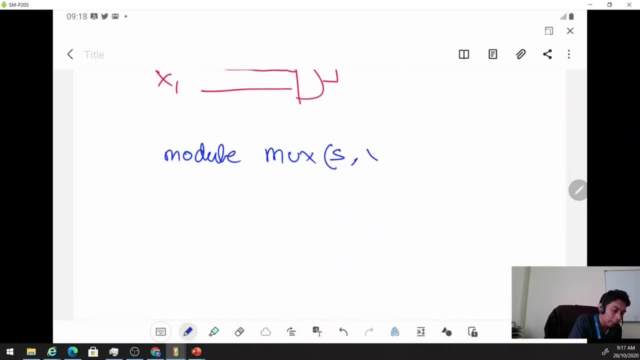 so you have f x 0, x 1 and f, right, and you need to tell your computer or software that the input is f and all the input are one bit input: f x 0. so if one bit input, uh, if like this, meaning that this is already one bit now, right, later, if more than one bit, we can. 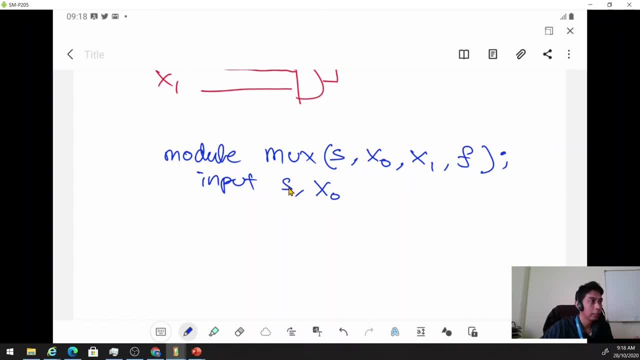 see, uh, we will see you what. how to declare all right the input or output for more than one bit: x, 0, x, 1, is our input done and we have one output with it, okay, okay, now we want to describe using data flow modeling. so the first one, data flow. 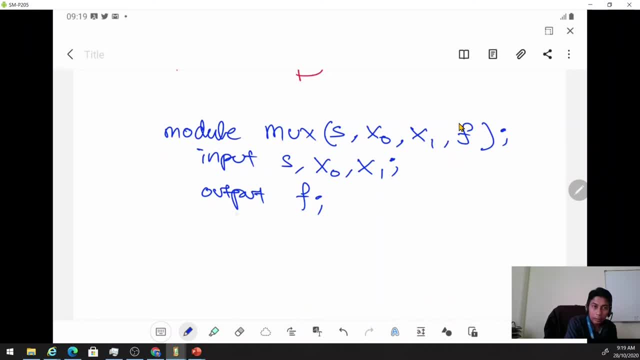 modeling. first you need to use the continuous assignment right, continuous assignment statement. so assign f. so that's f x 0 x 1 and f x 0 x 1. you also need to define f x 1- f 1 and f 2 x 1, f 0- f 1 and f 2- f 1. all right. so f i f x 0 x 1 and f 2 x 1 and f 1 x 1 f 0. you need to specify f x 1 x 2, f 1 x 1 x 2 x 1 x 1 and f 2 x 1 x 2 x 1 and f 2 x 1 x 1. so f 1 x 1 and f 2 x 1 and f 2 is equal to 4.. 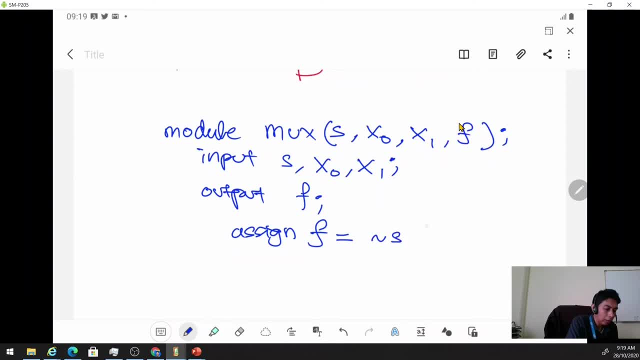 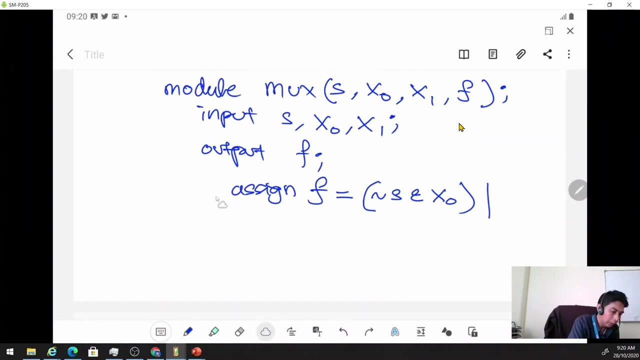 do. you don't have enough. sorry, you don't have enough space. okay, or so this is, or yeah, this is, or as n, as 1, right, and I'm done. Okay, So this will be data flow modeling. alright, and you do this data flow modeling and also. 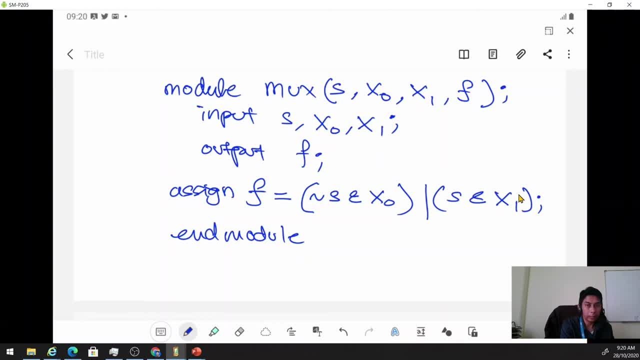 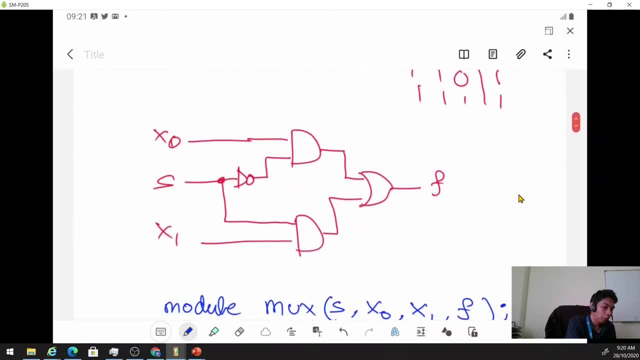 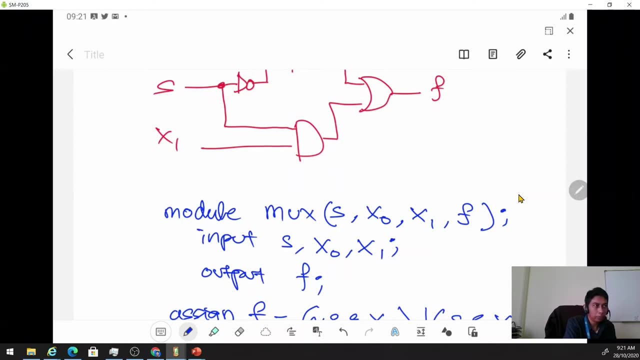 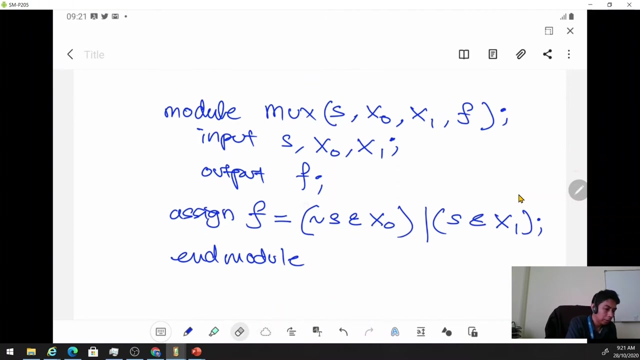 you can describe your circuit using behavioral modeling. So how to design a circuit using behavioral modeling, right name and go on. and you need to know the behavior of the circuit. okay, so let's see, we want to, so here should be the same. then one more: to model using behavioral modeling. so 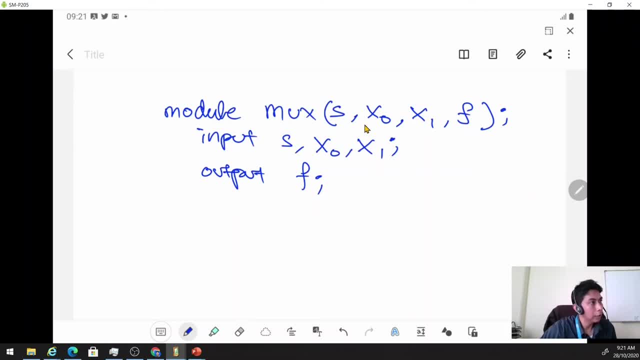 the module. the name should be no problem. yeah, the input list, the port list should be no problem. the input should be no problem and f should be no problem. all right, the output is still the same. now, when you want to describe using behavioral, what you need to use is you need to use sequential. 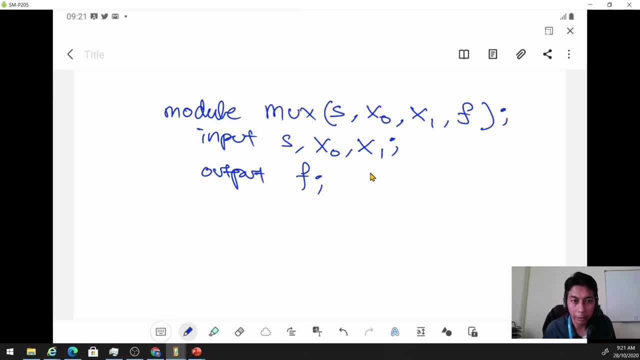 assignment statement. and when you want to use sequential assignment statement, you need to use what we call an always dot. all right, so always how to how to use obvious dot. this is how you write always lias, and here we call yeah in the bracket, here we call sensitivity list. 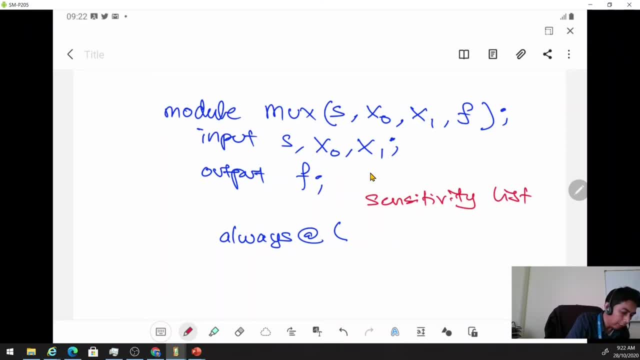 sensitivity. so what is sensitivity least sensitive, sensitivity least is the signal? all right, that is signal, because we want to, to, to observe. f right, the output is f. the output is f. so what is the input or what is the signal that will change f? all right, that effect. 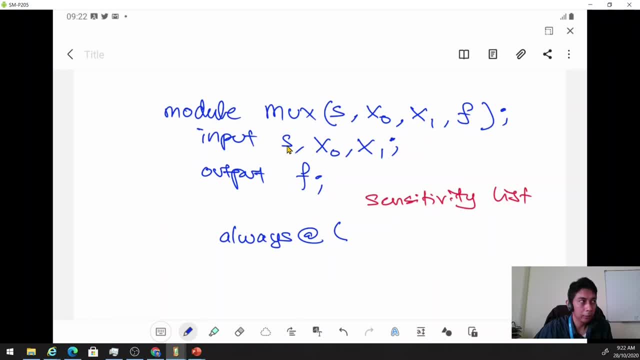 f right. for example, here we know that the, the signal that will affect f is s, x, 1, x 0 and x 1, right, so this signal must be inside sensitivity x 0. the way you write is like this: you can have a comma, or sometimes in the textbook, sometimes you. 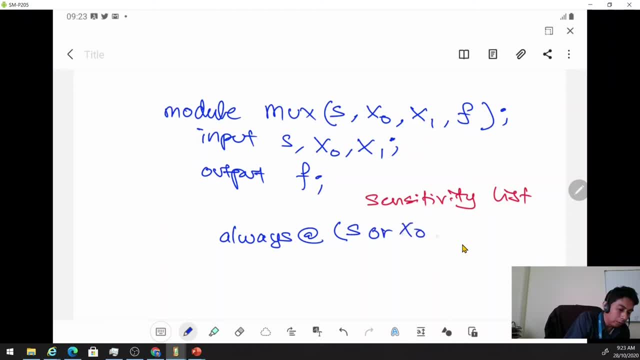 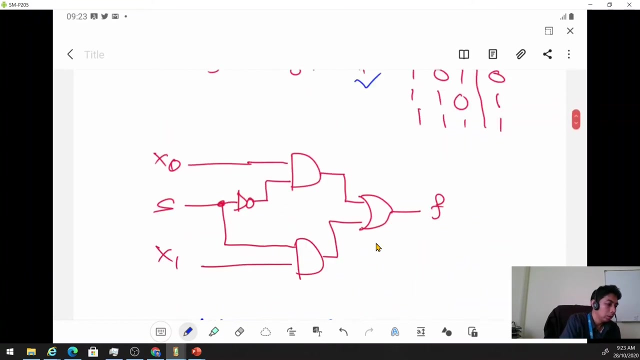 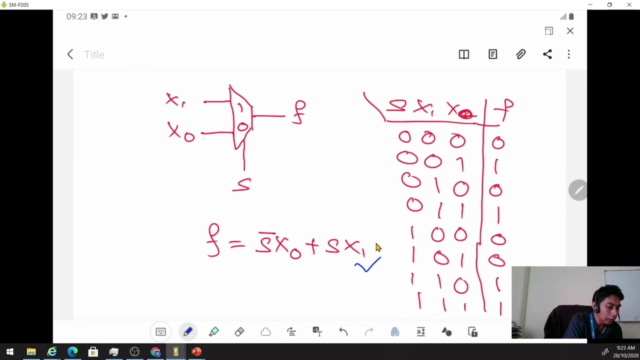 use 4 x 0, 4 x 1, 1. all right, you can use comma to the base all also can, no problem, all right, but we need to know that this is what we call sensitivity list. so this is because whenever one of this signal and one or two of all the signals here, all right as x0 or x1 change it. 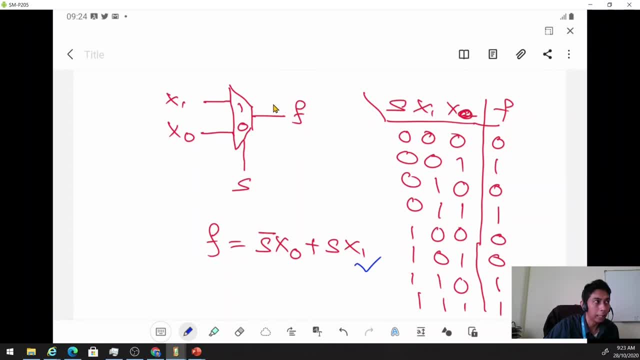 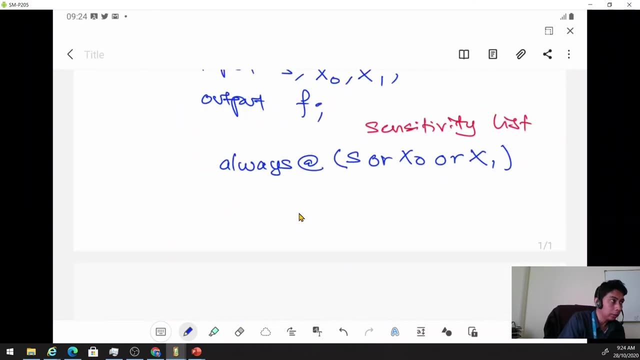 will affect f. it will make the f change value. right. so this three signal now we call sensitivity list must be inside the sensitivity list, okay. so what's so good now in the always block? yeah, if you have many statements, all right, you need to have begin and end, and your statement is should be inside, inside this. but if you have only one statement, 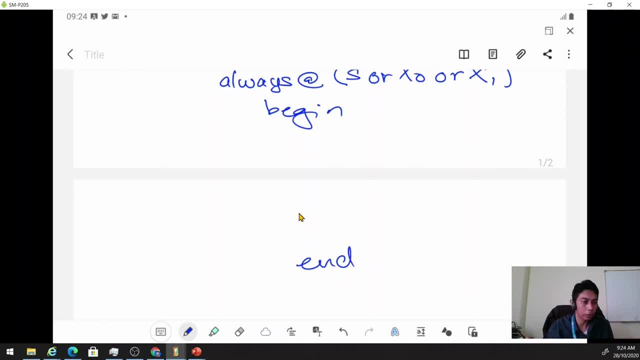 means that one, only one line of of code, so no need to put begin and end. all right, just like c programming. now, if you have many, many, uh, many lines of code, right, so you need to have a calibrated bracket and then close, calibrated, right same thing. now, how to describe this circuit? so by using behavior. you need to. 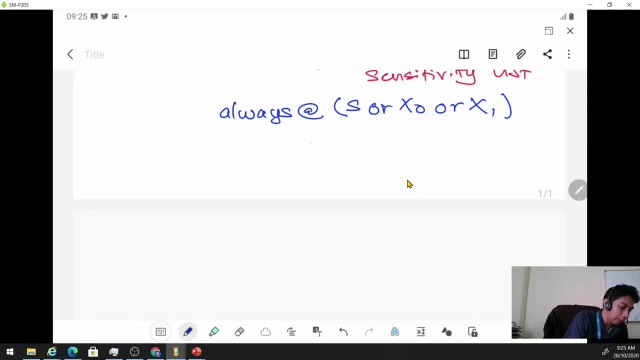 we can use if and else statement. so we can write like this: if s equal to zero, yeah, f should be equal to what? if f equal to zero, f should be equal to x1. right, so f should be equal to x1 here. but if s not equal to zero, or we call: 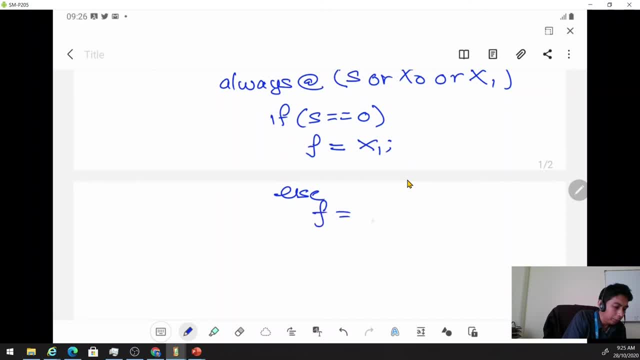 s not equal to zero, or we call s not equal to zero, or we call l. that should be equal to zero. but if f equal l, that should be equal to zero. but if f equal l, that should be equal to zero. but if f equal to 1, f should be equal to x1: all. 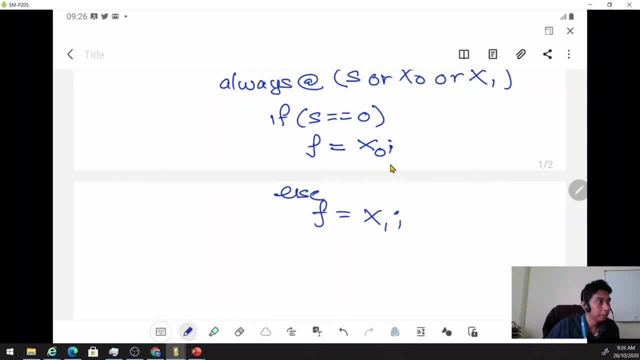 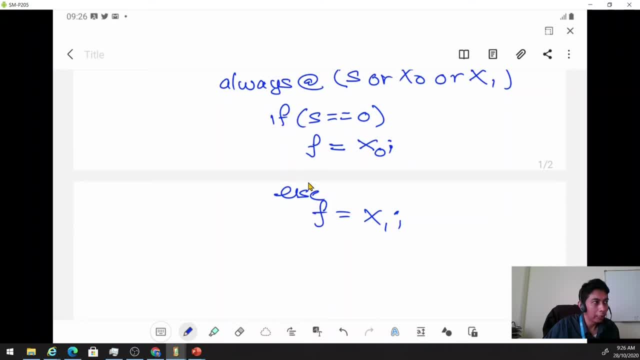 all right, this is question for you. i have all right, this is question for you. i have all right, this is question for you. i have many lines, of many lines, of many lines of of code here. do we need begin and end here? anyone want to answer so? 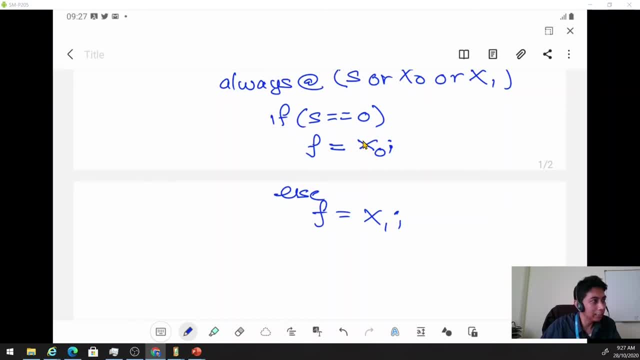 anyone want to answer? so? anyone want to answer. so the question is that, if we have many, the question is that, if we have many, the question is that, if we have many lines like this, lines like this, lines like this, if this do this, else you do this. 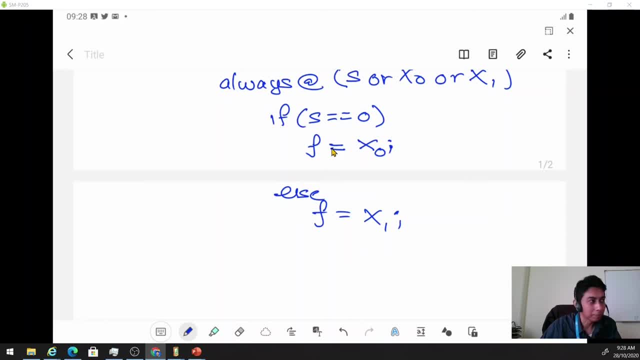 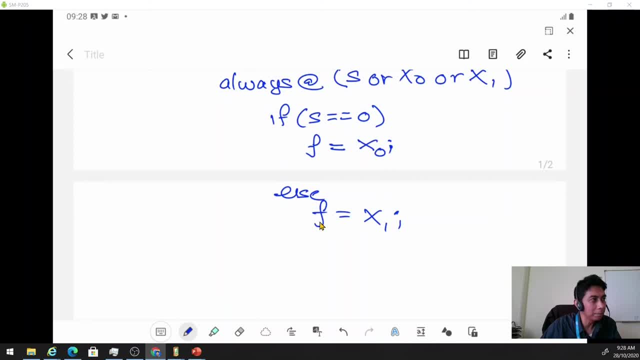 look like other one line, look like other one line, but but but this statement is the same statement. this statement is the same statement. this statement is the same statement. they continue, they continue. they continue from from this, this, this and else this. from from this, this, this and else this. 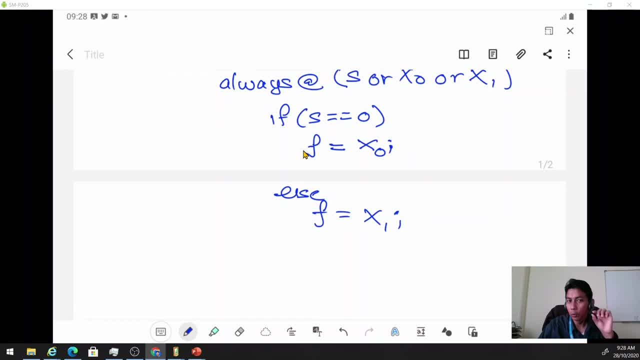 from from this, this, this and else. this means that this is considered, means that this is considered, means that this is considered one one statement, all right. but if you one one statement, all right. but if you one one statement, all right. but if you have another statement, for example, if 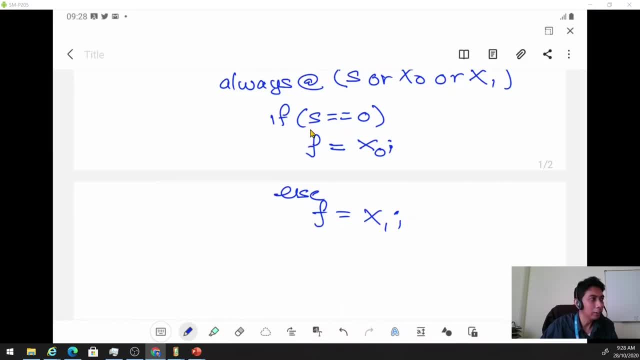 have another statement, for example. if have another statement, for example, if like this, like this, like this, sorry if then you need to begin and sorry if then you need to begin, and sorry if then you need to begin and end. but if only one if and else no need, all right. that's why i 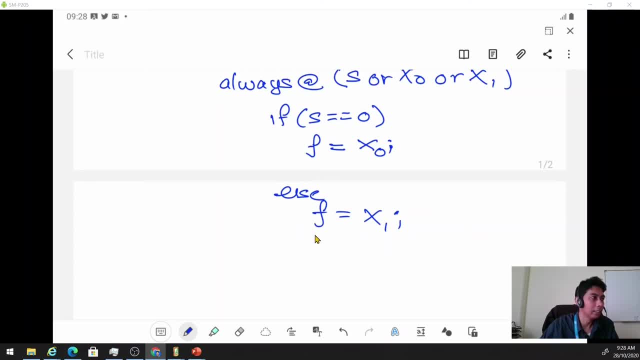 no need all right. that's why i no need all right. that's why i i don't read, i don't write begin and end. i don't read. i don't write begin and end. i don't read. i don't write begin and end here here. 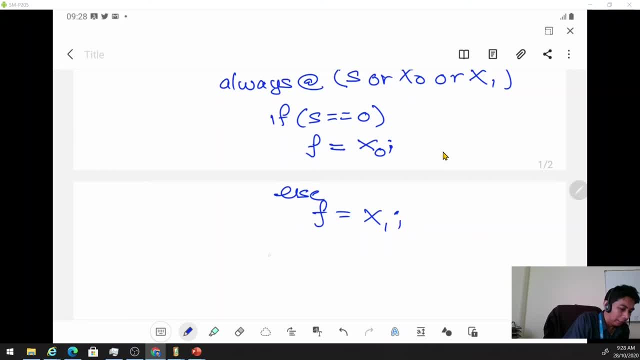 here: okay, and and, and. this is done, so you can, this is done, so you can, this is done, so you can module. okay, okay, okay. so this is behavior, so this is behavior. so this is behavior, all right. so, if you design your circuit, all right. so if you design your circuit, 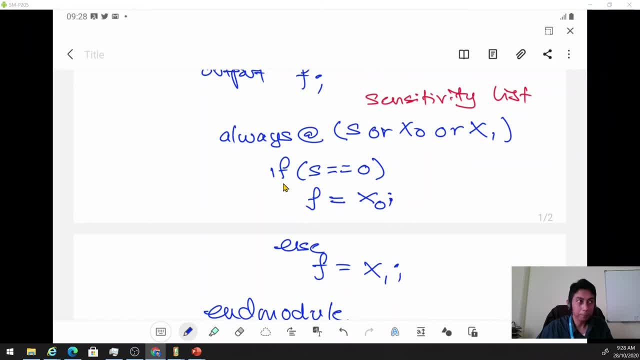 all right. so if you design your circuit or you write the code for your circuit, or you write the code for your circuit, or you write the code for your circuit like this, like this, like this, if, if, if this you do this, else you do this. this is the behavioral. 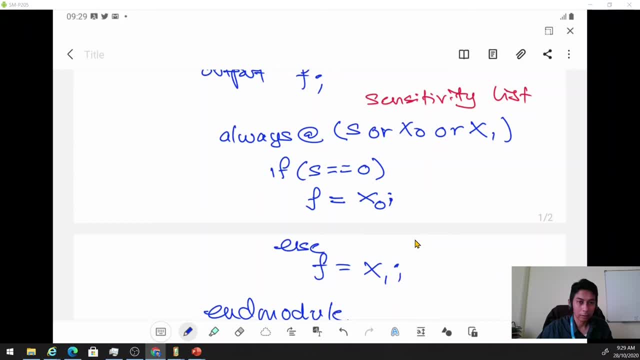 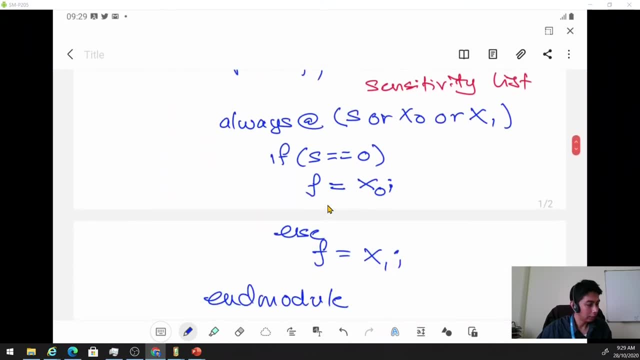 this is the behavioral, this is the behavioral modeling. all right, i hope you get that. all right, i hope you get that. all right, i hope you get that. but if you use, but if you use, but if you use boolean equation, boolean equation, boolean equation, that is, that is. 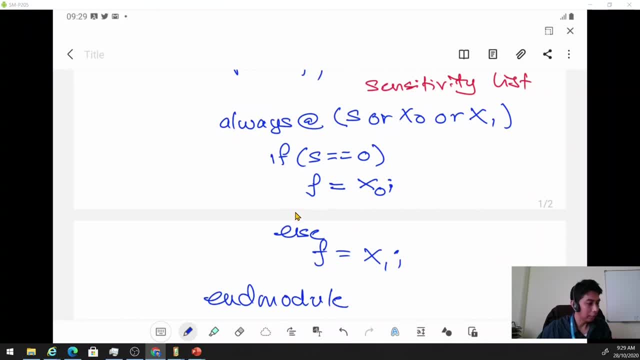 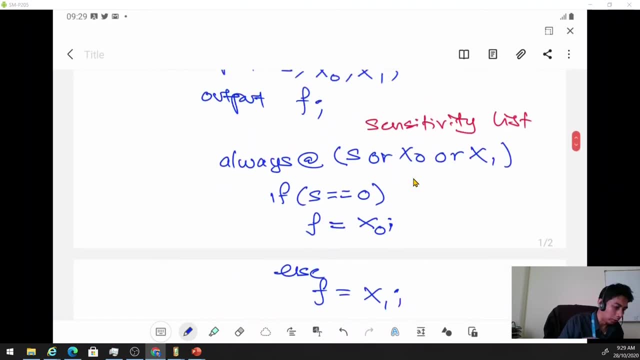 that is, data flow modeling. data flow modeling, data flow modeling- all right, the last one. all right, the last one. all right, the last one. structural modeling, structural modeling, structural modeling, sending. oh one more thing, oh, one more thing, oh, one more thing. this is not finished yet. this is not finished yet. 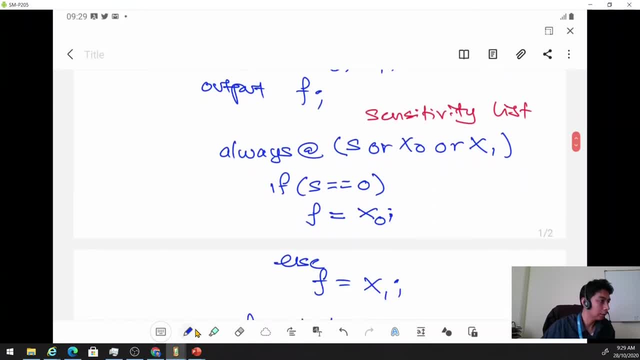 this is not finished yet. all right because. all right, because all right, because now, because you have, you have, you have f. here you assign a value to f. f. here you assign a value to f. f. here you assign a value to f. remember this: when, whenever you assign. 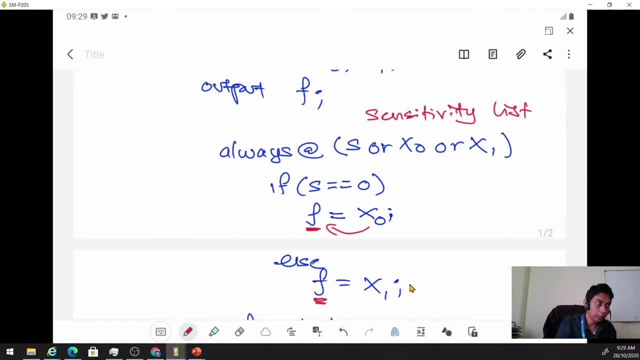 remember this when, whenever you assign, remember this, when, whenever you assign any value, any value, any value to uh, to uh, to uh, f or to any any uh, any variable like this f. or to any any uh, any variable like this f. or to any any uh, any variable like this: all right. 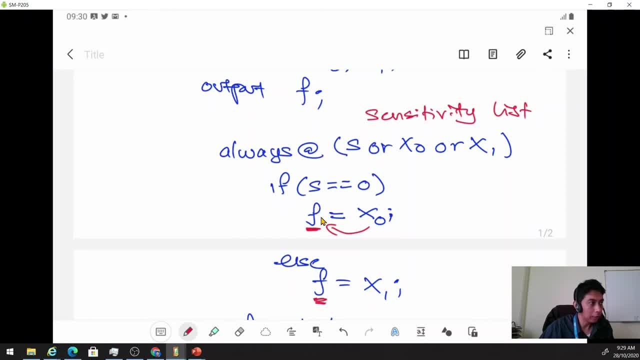 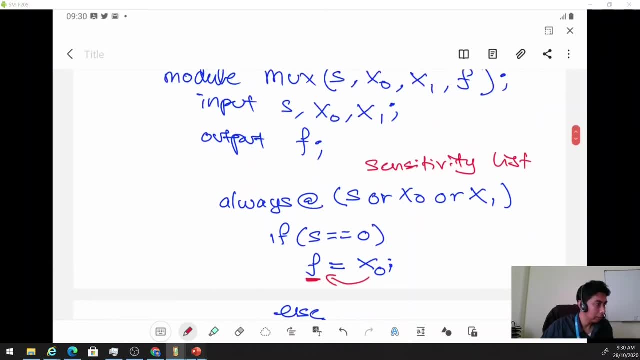 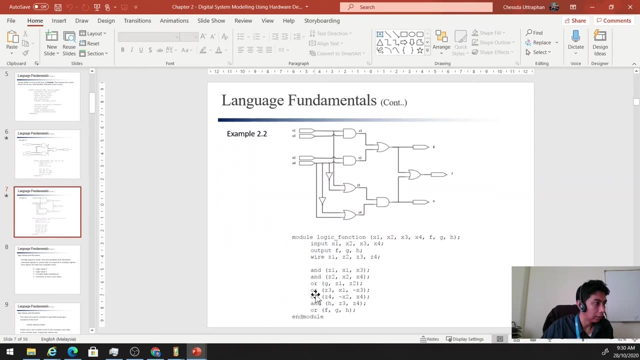 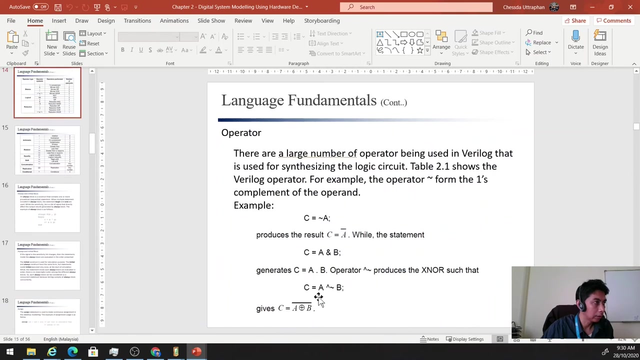 all right, all right, you need to declare, you need to declare, you need to declare. this variable, in our case is f s r. this variable, in our case, is f s r. this variable, in our case is f s r right, right, right, remember, Wrecked, correct now, yeah. 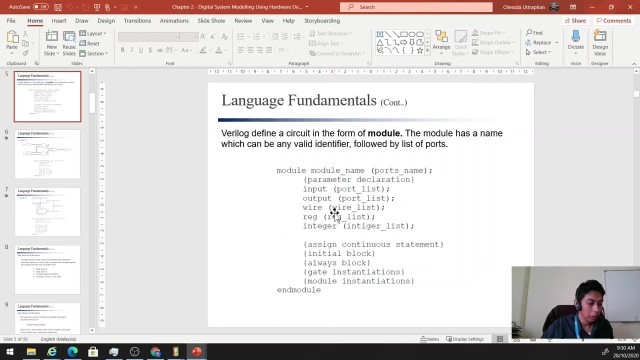 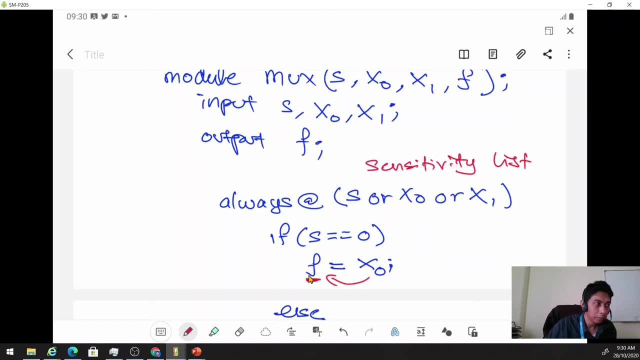 correct now. yeah, correct now. yeah, r e g right please. r e g right, please. So whenever you assign any value to a variable inside always law, you need to declare that variable as right. So right here, right F, Alright, and F is the output. this is correct already, so you need to declare 2.. 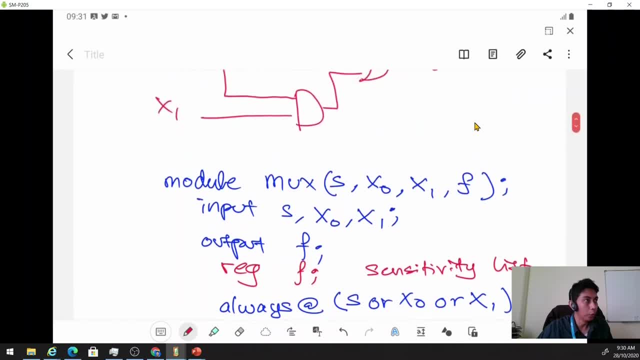 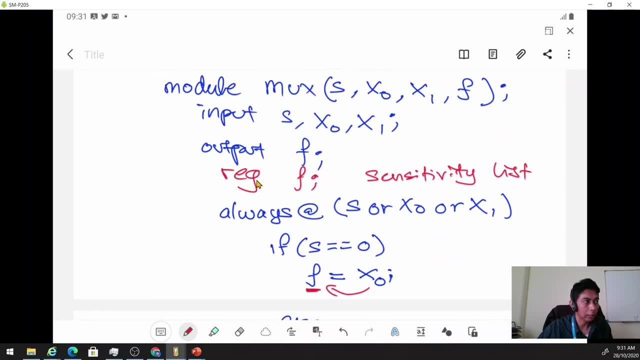 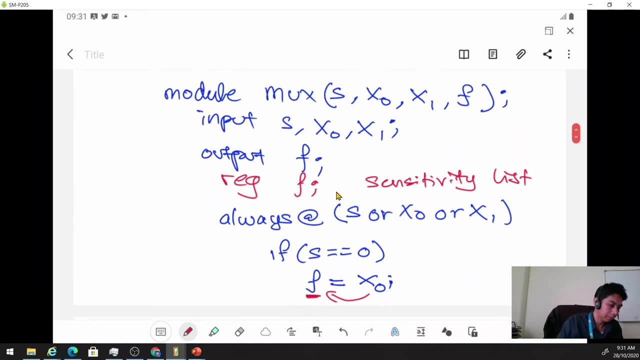 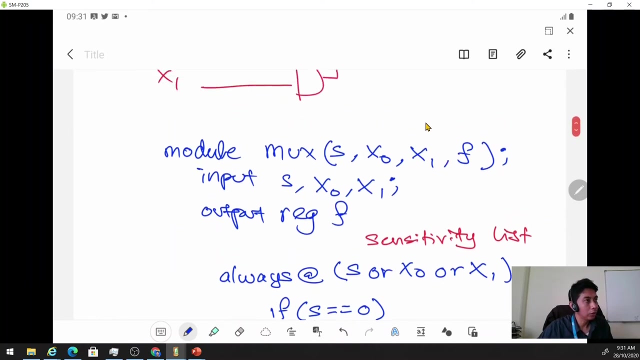 F also as an output and F also right, right, R-E-G. so remember, alright, or you may write like this: you may write like this: output: right, F, right, because F is right, right and also an output. alright, now the code is complete. 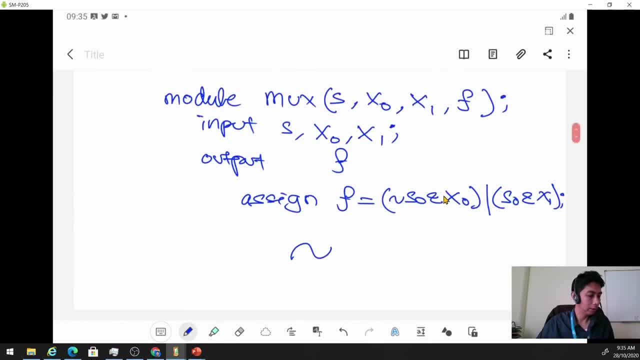 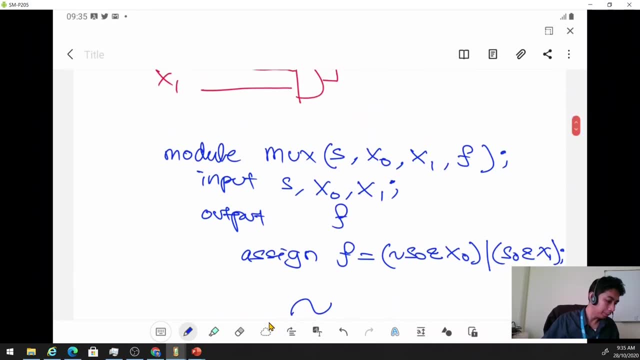 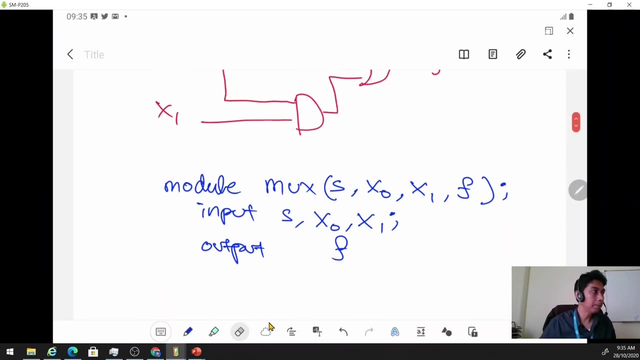 So this we call behavioral modeling, alright. and the last one is the structural modeling. So, structural modeling, right, it is used to describe the same, the same circuit actually, but what you need to have, You need to have the. 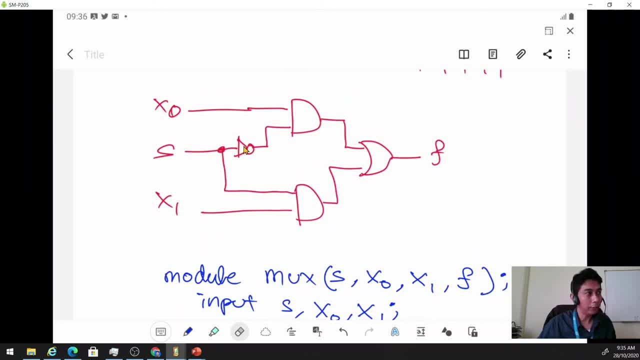 The schematic, and now we have the schematic. right, we have the schematic, so we can describe this using gate instantiation, because we have- yes, this is N-gate- connect to this. the output is this: this is the OR gate, NOT gate. it should be no problem, right? and 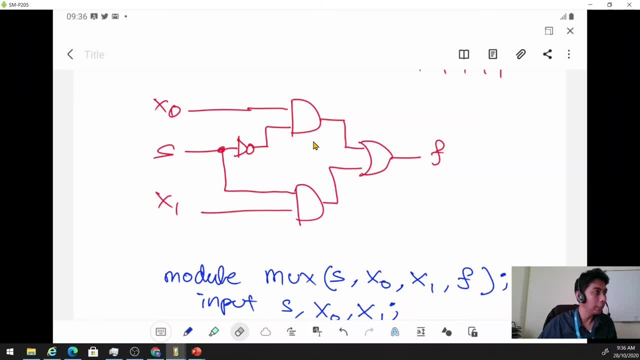 the signal. we have already so, but we have internal internal wire. yeah, so you need to name the internal wire in order to To use the gate instantiation, Right? So this one, let's name this wire as A and this one is C so that we can instantiate. 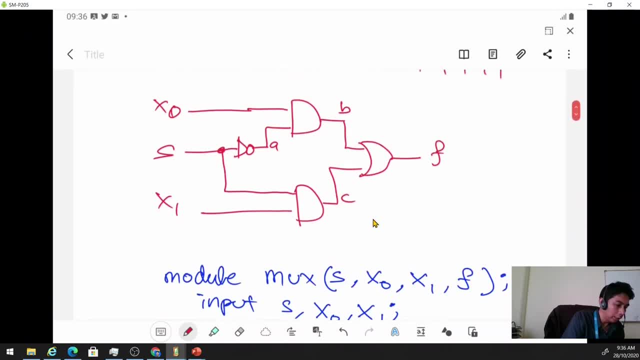 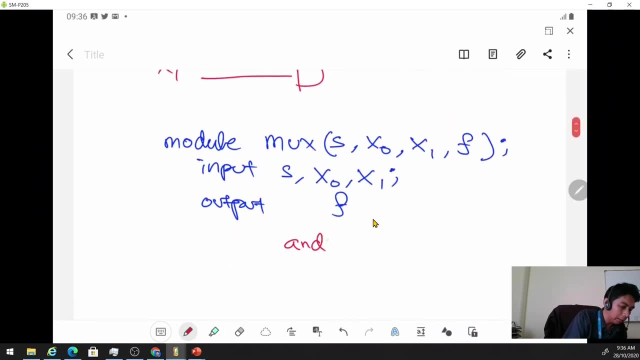 the module. yeah, So how to instantiate the module? Very simple. for example, we start with this, this gate, so we can have N. what is the output? N, Okay, What is gate Should be? Should be B. 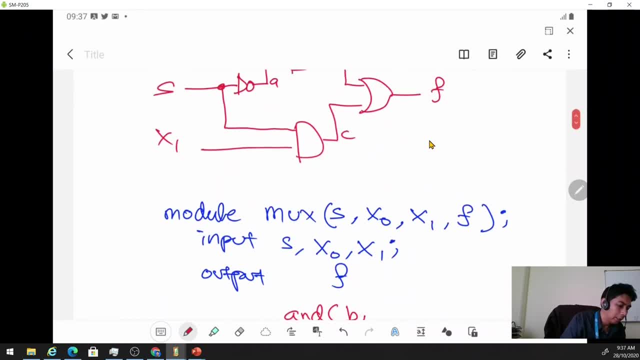 Right B, And the input is X0 and A. So X0 and A, Then the first gate, The second gate. maybe we want to describe this, but this is NOT NOT. And remember, use small letter. 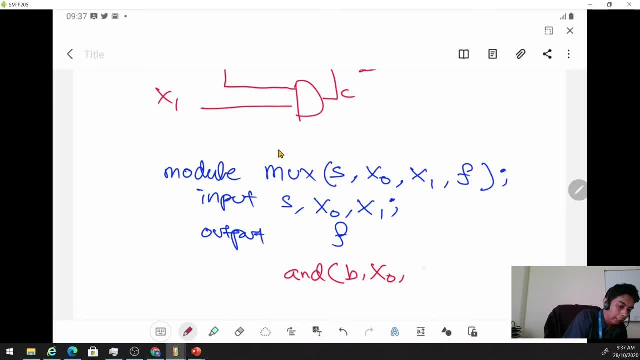 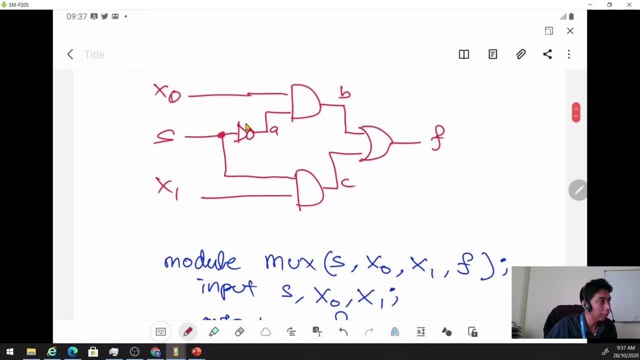 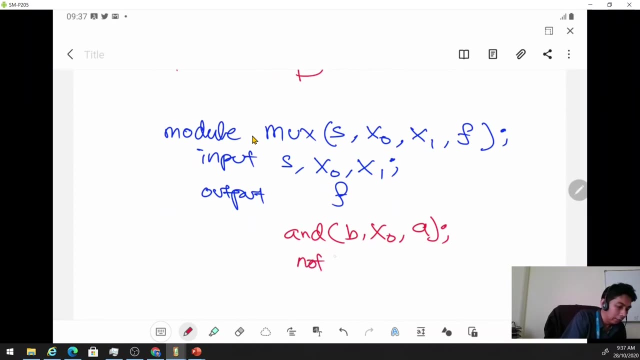 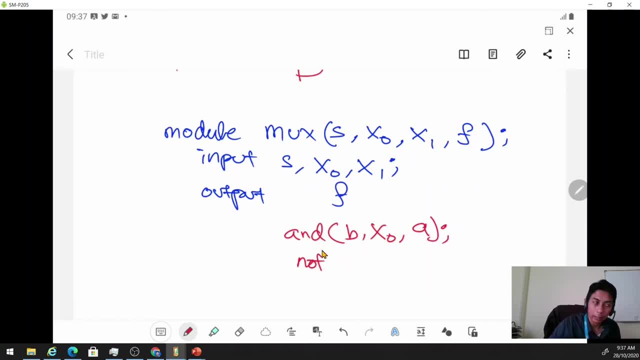 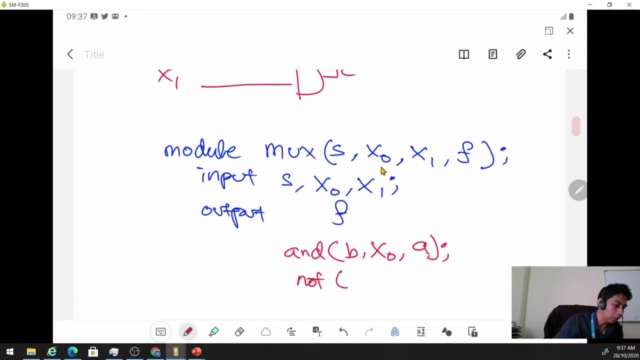 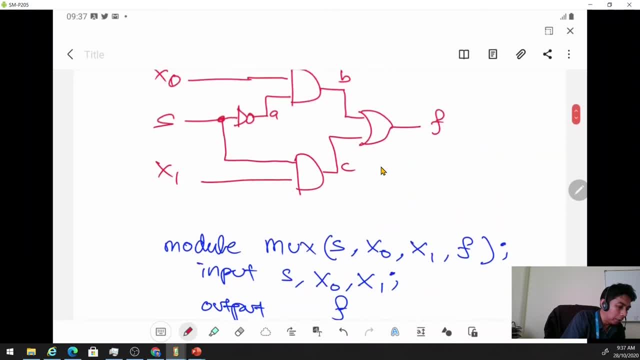 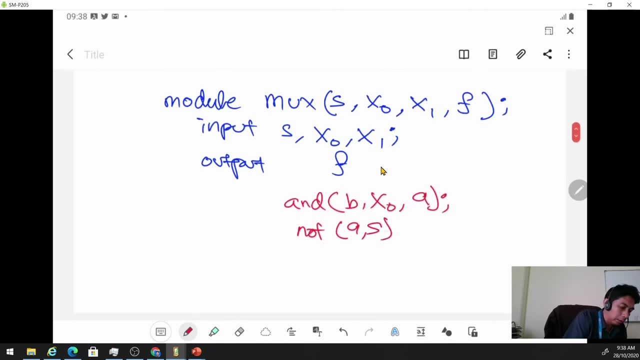 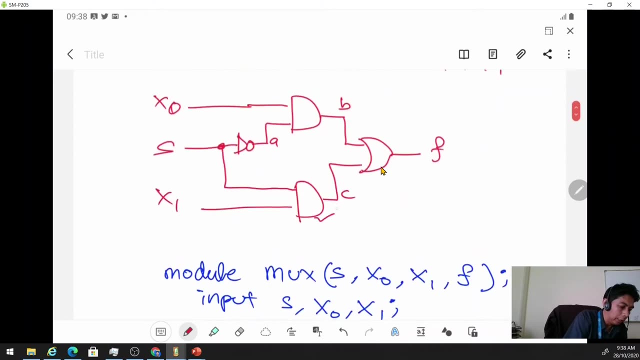 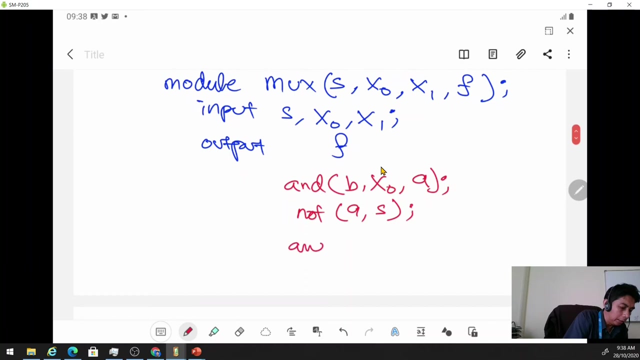 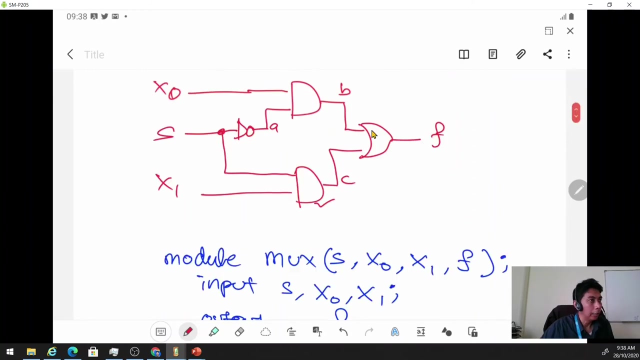 Yeah, Now we will take this to another level, to another. How often? ah, yes, yeah, the input is c, s and x1. so, and uh, output is c, s and x1. okay, and the last is the object: f, b and c. so all. 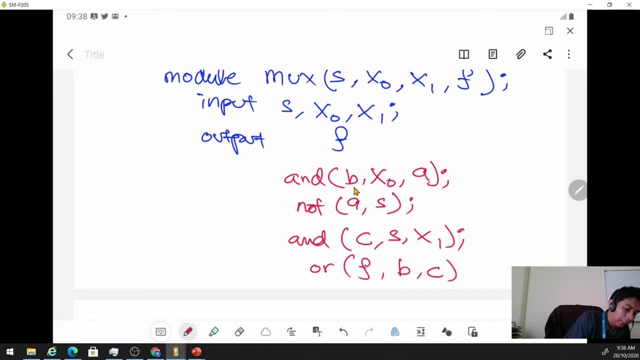 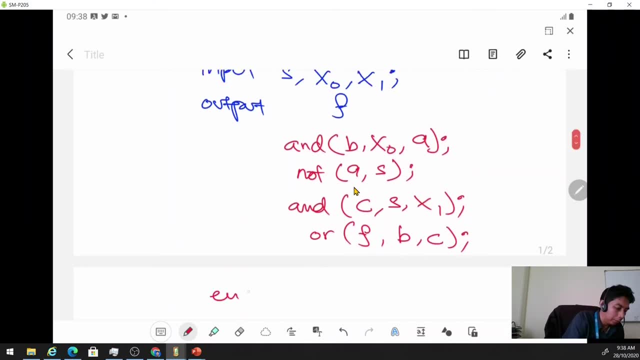 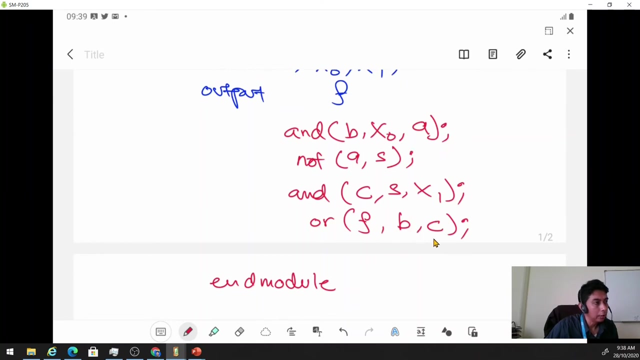 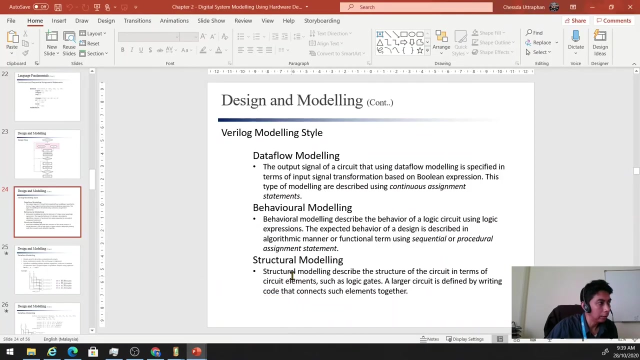 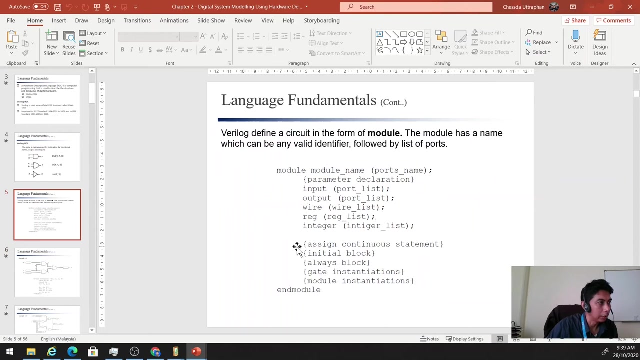 f, b and c. right and this is done and model, but don't forget, because we have additional signal right- a, b and c- so we need to declare this as a, as a. what as a input? declare as a this, this is, this is, this is in the 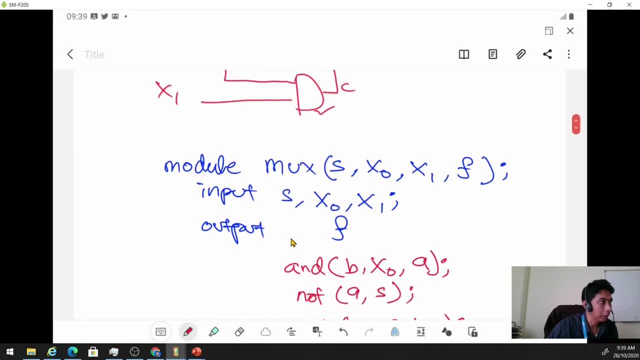 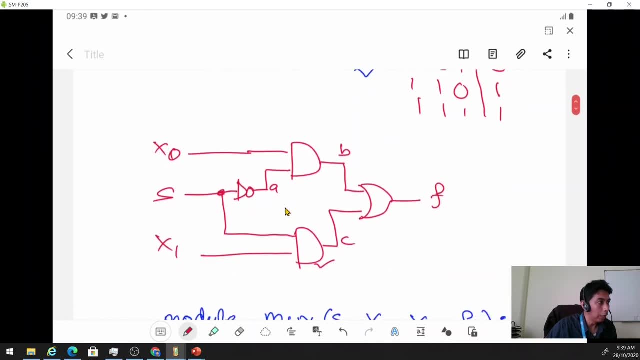 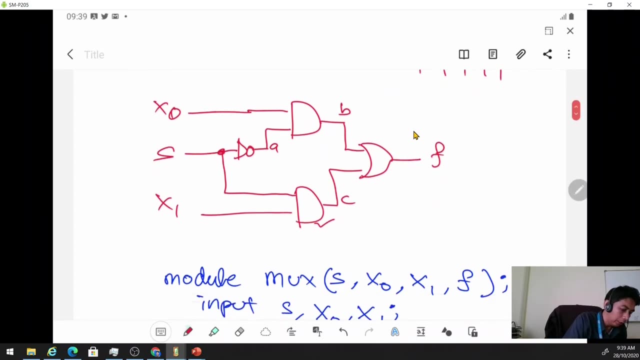 ah, warrior right, because it is internal and this is not input or output. a is not input, output of of your. i mean, this is not input or output of your module and your, your module, your module is this: you need, you need to understand this. your module is this: 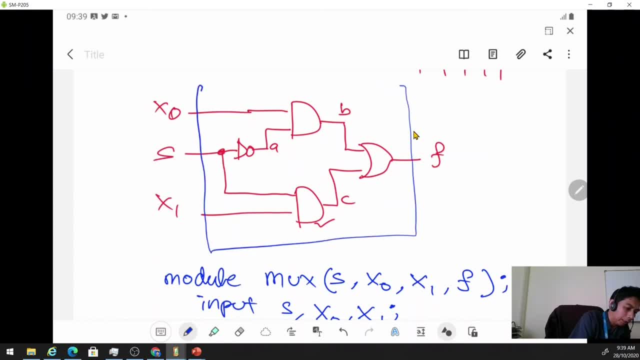 this is your module, the all right. so, input or output, is this input, input, input, output. but here here, here is not input or output of your module. this will be wire, internal wire of your module, right, so so? so you need to declare this as: so you need to declare this as: 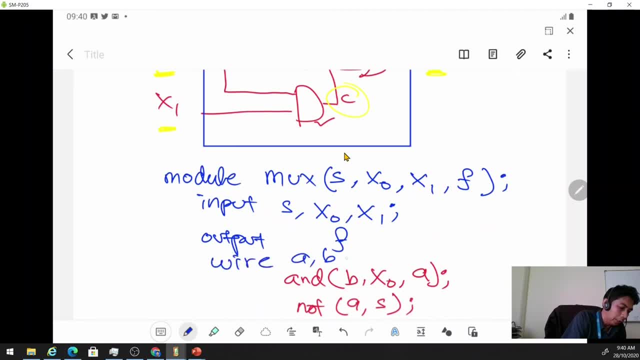 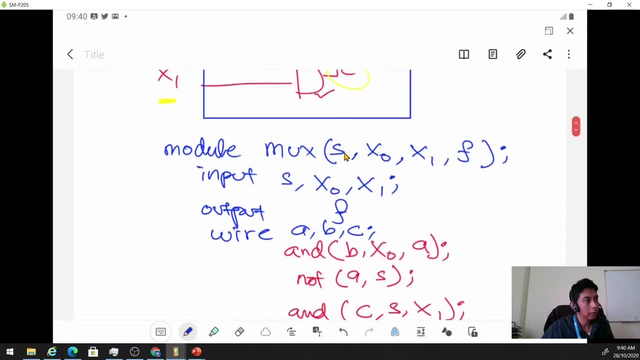 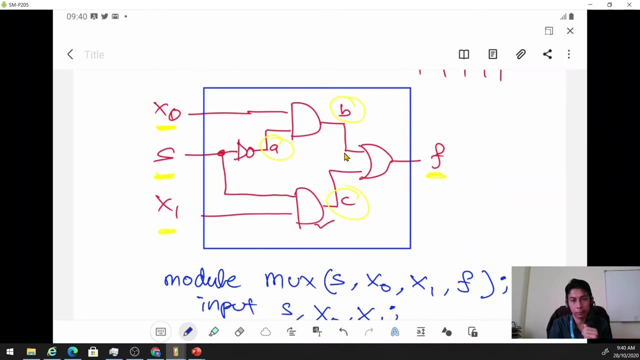 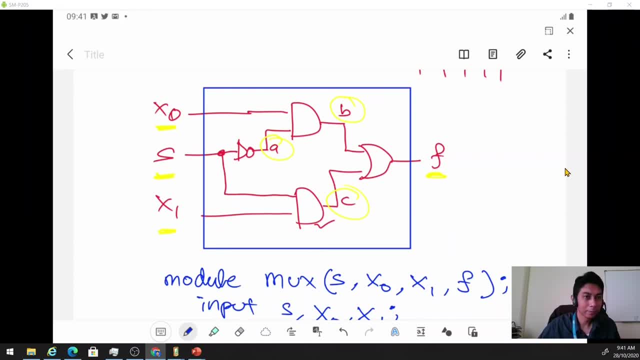 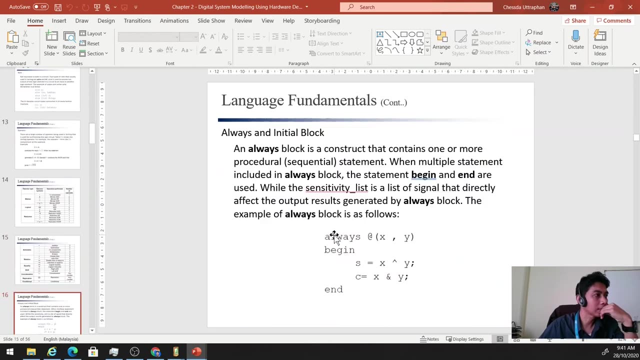 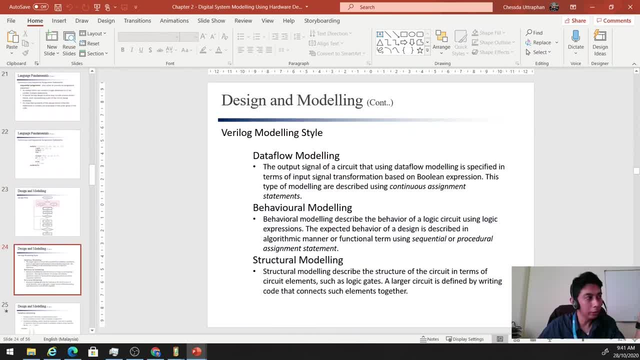 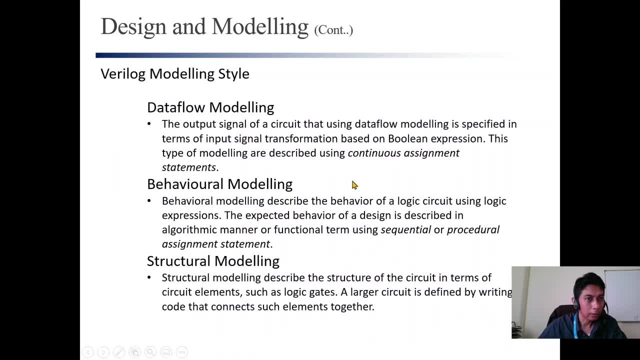 in very low. all right, all right, all right, so again, so again, so again, uh, uh uh. we have data flow modeling. we have data flow modeling. we have data flow modeling. when you have, when you have, when you have boolean equation, then boolean equation, then boolean equation, then you have a problem. very fast, right. 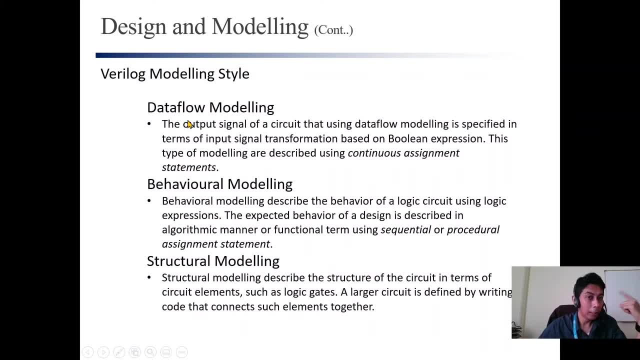 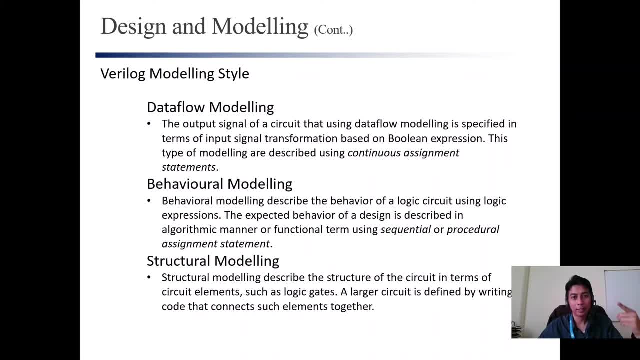 when you, when you design your circuit, when you design your circuit, when you design your circuit, a complex circuit, a complex circuit, a complex circuit, a big circuit, a big circuit, a big circuit. all right where the input is more than. all right where the input is more than. 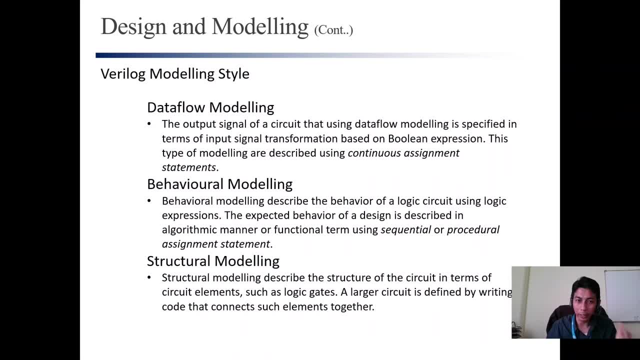 all right, where the input is more than more than 5, 10, 20, for example, more than 5, 10, 20, for example, more than 5, 10, 20, for example, and the output is, and the output is, and the output is 20 or so. 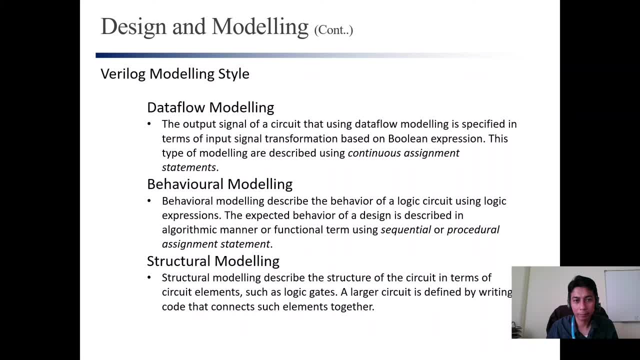 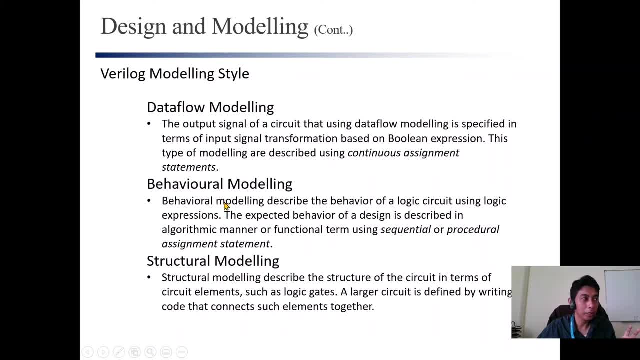 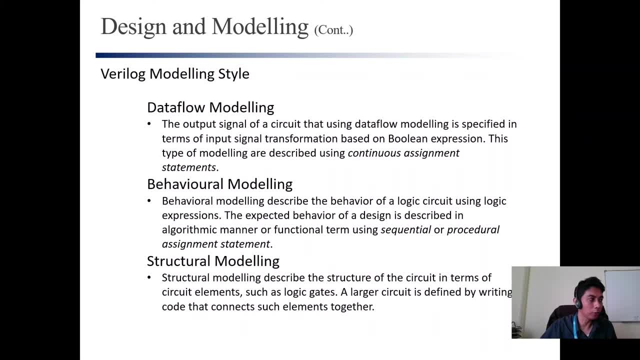 and we don't have the schematic. of course we cannot do structural modeling, except that you want to connect your sub-module, Your sub-module, okay, no problem. So there will be a limitation for each modeling style. So for the bit circuit, for the actual circuit later on. 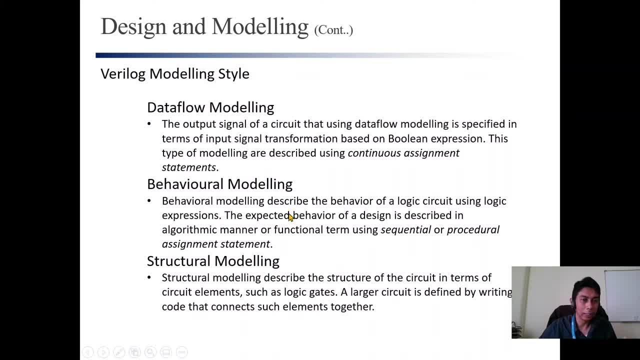 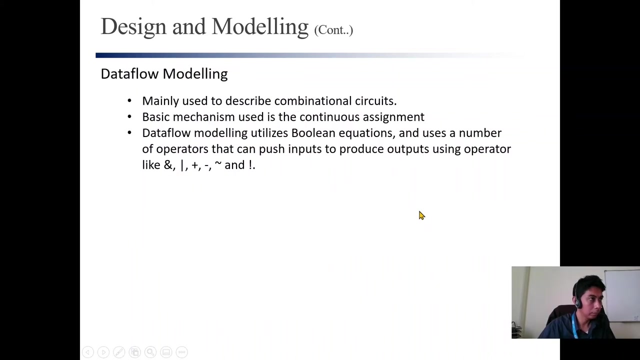 you may combine the modeling style in your design. Sometimes, for example, you want your design the bit design like this you have here, which is quite big, and this is there are many logic. things are here all right instead of oh sorry, all right. 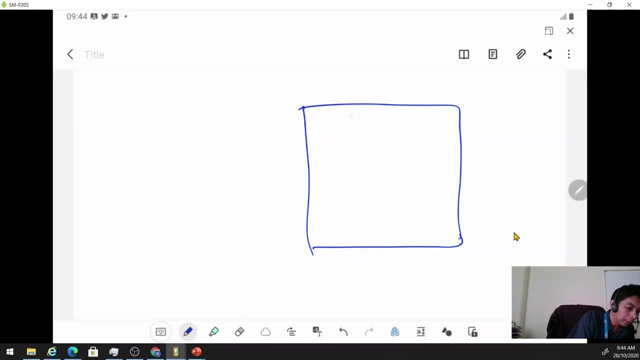 So, for example, you have a complex- ah, complex- design here, A lot of gif, a lot of logic inside here, But one of the signals here- all right, one of the signals here is come from a simple, simple, simple. 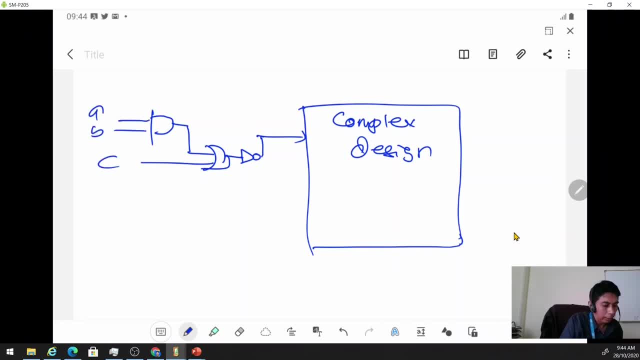 okay, like this, all right. So this, for example, this signal is Y. So here, to provide this Y signal to this, you can use the data flow modeling to get Y. And here maybe you need to describe using behavior. 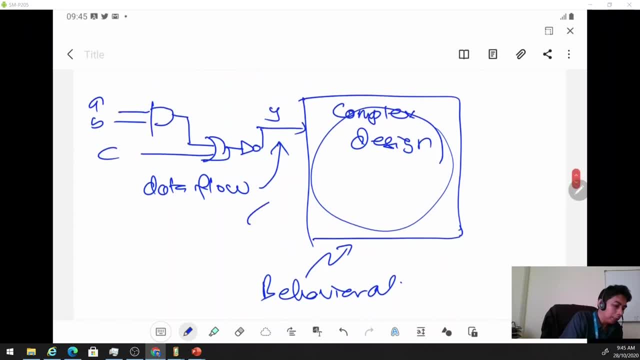 all right, And some of some of the connection inside. maybe you want to connect your sub modules inside here. This one is connected to this. this one is connected to something like this. right Here you may use structural modeling. 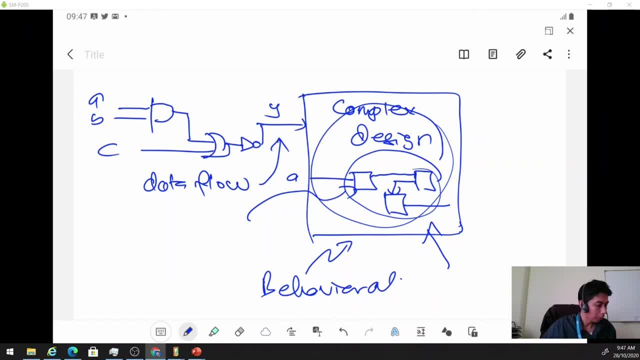 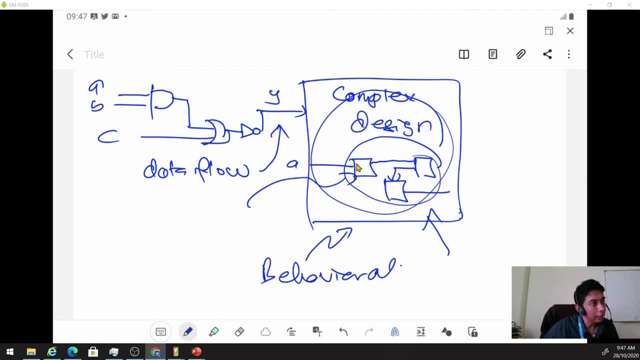 All right. So again, if you have a sub module inside your design here and you know the connection, this module should be connected to this module. this module should be connected to this module and this one is for the output, for one of the output. 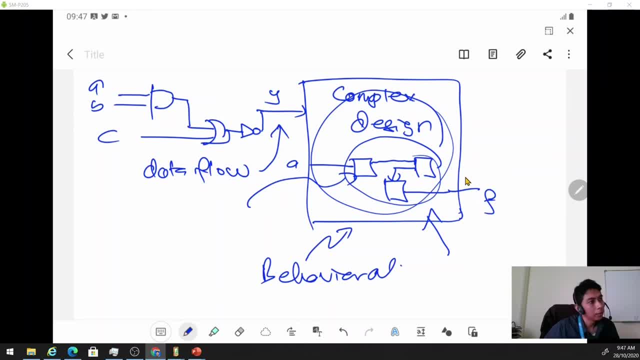 for example, this one is F and you have many more. all right, So the connection like this: you can use these structures. okay, So in your design you may have three kind of modeling. All right, The combination of all the three modeling styles. 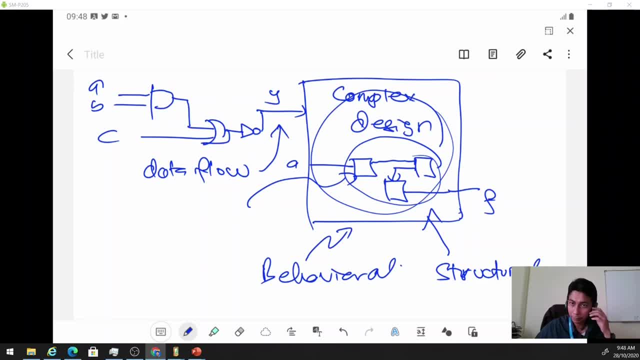 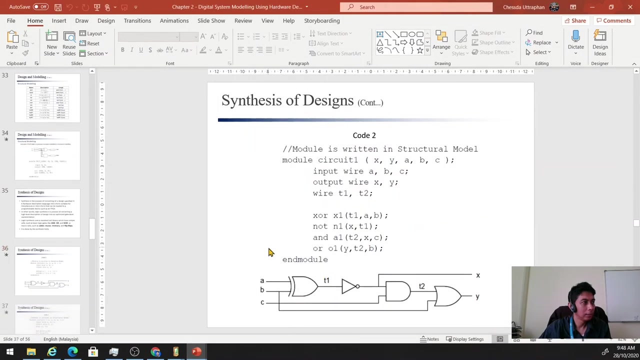 All right, So can. the answer is: can, Okay, All right, Dewa. Okay, You can, And of course you can do that. Yeah, And of course later we can do that, Okay. Any other questions? 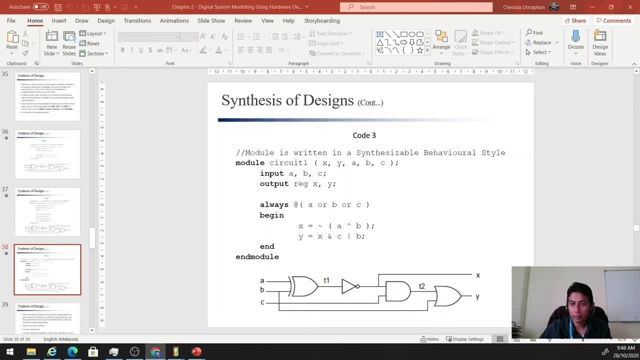 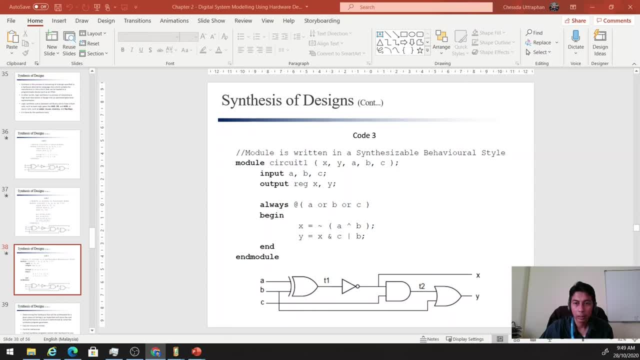 Thanks you, Thanks you See you guys. bye, Bye, Bye-bye, Bye-bye, Bye-bye, Bye-bye. Yeah good, See you later guys. See you later guys, Yeah good. 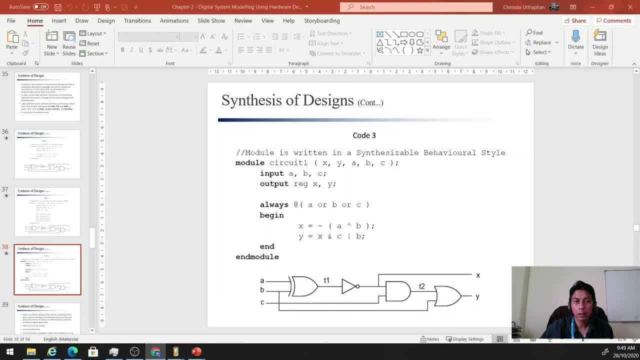 All right, See you later, guys. Bye-bye, Bye-bye, Bye-bye, Bye-bye is according to the logic gate. what do you mean? according to the logic gate, no truth table is. according to specification. truth table is according. 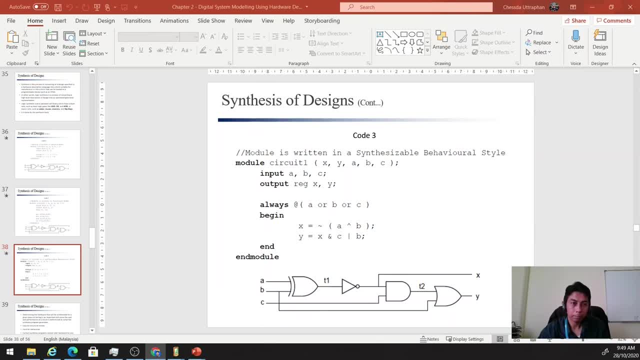 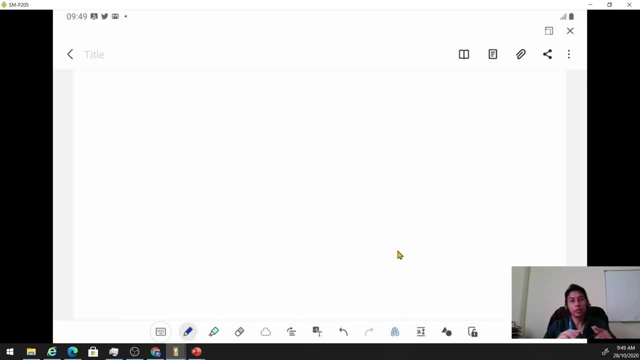 to specification. for example, all right, for example, you want to design a very simple alarm system, all right, office alarm system. this is the office for floor plan and, for example, we have three doors right. the number one, but mainly this one, is b1 the term and this one is b3. so let's say we, we want. 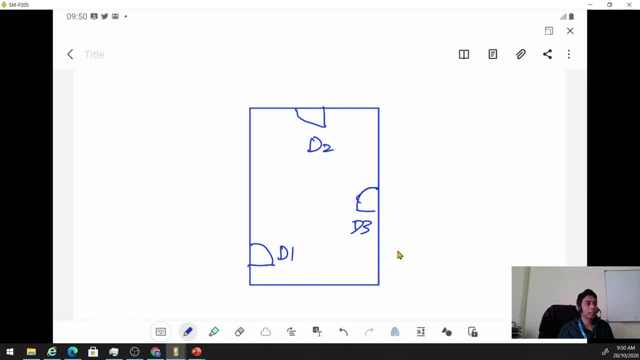 to design a system that can detect now if two or more doors is open at the same time. right, you get what i mean and we have an alarm here, okay? so, for example, if door one only open at one time, door one open and door three and door two is closed, so the alarm will not. 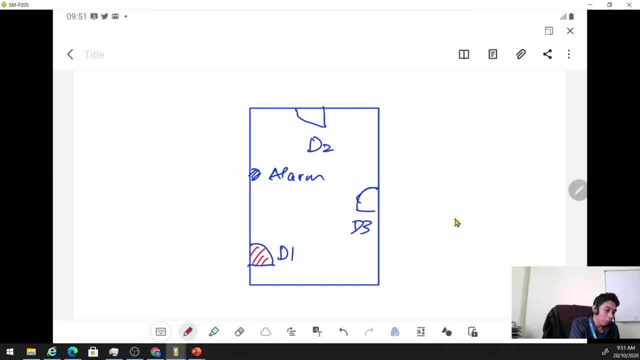 will be not activated. but if door one and door three is open at the same time, alarm activated, or door two, door three open at the same time, alarm activated, or all the doors are open at the same time, then the alarm will be activated. that will be the specification, right? so, uh, the true stable will be derived from this specification. 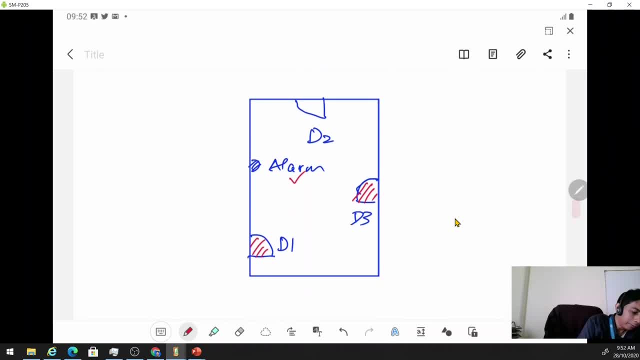 so in this case, so we can have something like this to stable, right, you can have a table like this. so what are our input feature b, 2, d, that and the output will be the alarm then and what are the combination, the possibilities. so we have how many possibilities? because we have. 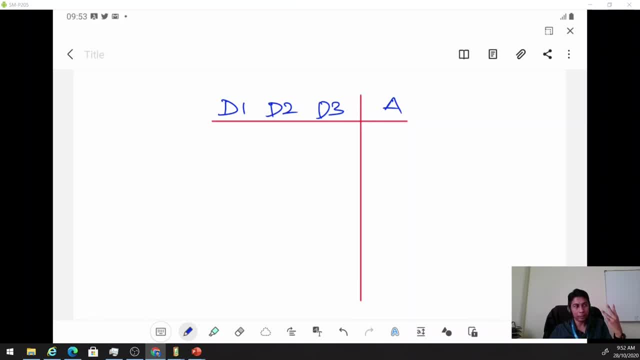 three input, so the possibilities should be eight. two power of three, right. so we have three possibilities, eight possibilities. the first of possibility is on door. for example, if zero represent uh door close, one will present open. so all doors are closed, so the output will be zero. the alarm is not activated, all right. and if one door is open, door number. 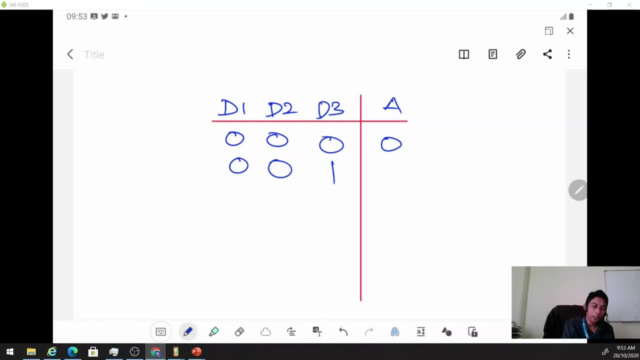 three. d three is open, so the alarm will not be activated for so and when? when d two is open, not activated, but now zero, one one. two of the doors are open at the same time. this one is activated. okay, and one zero. zero is one. no one, zero one. yes, one one, zero, yes, one one. 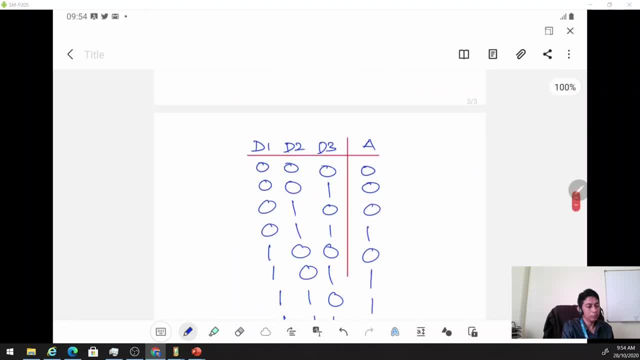 one. yes, okay, so this is the truth table. right, so this is the truth table. so from the truth table you can get the. you can get the boolean equation, all right, all right, so can you get the boolean equation for this? can you get the boolean equation for this? of course, yes, right. 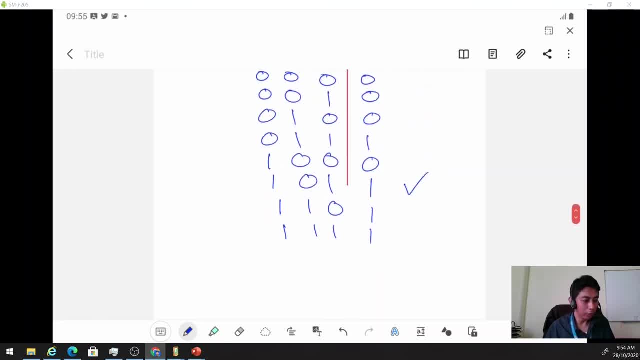 so here, if you have this now, you can. you can. you can describe your circuit using using what kind of modeling data flow can or not can? and because you can get the boolean equation: behavioral can what? huh? no, no behavior, no need to draw the logic. yes, yes, you can. you can, you can write if else. 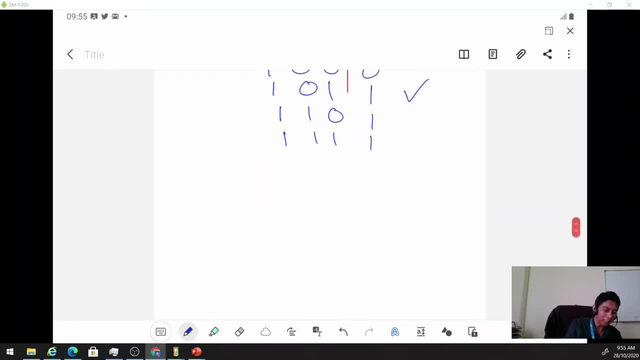 yes, yes, you can, you can. you can write if else. yes, yes, you can, you can. you can write if else, and so you can. you can say something like this: and so you can. you can say something like this, and so you can. you can say something like this if: 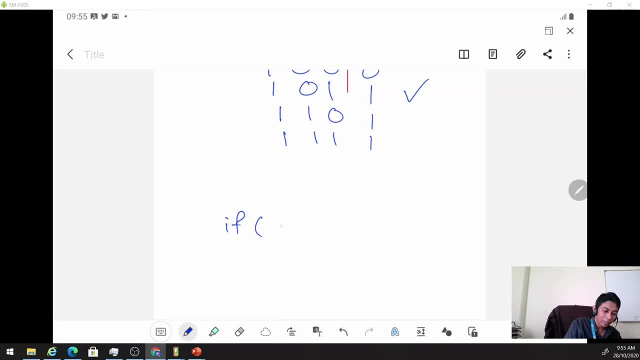 if, if, yeah, yeah, yeah, if d1, d1, d1, and now here and now here and now here. you use double n now, what logical. because you use double n now, what logical. because you use double n, now, what logical. because we want to test. we want to test. 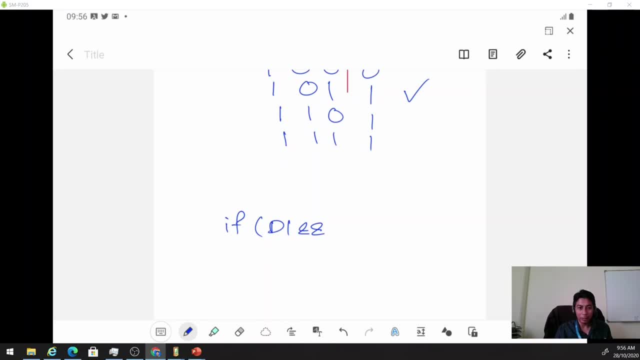 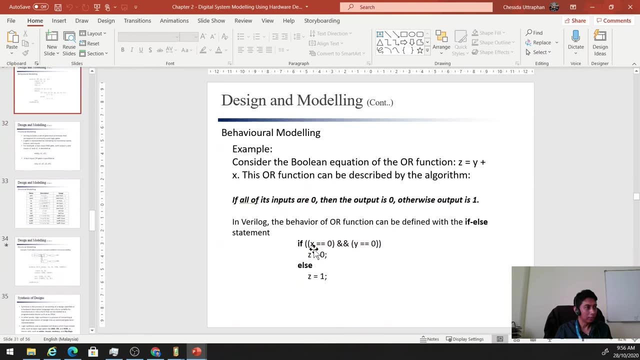 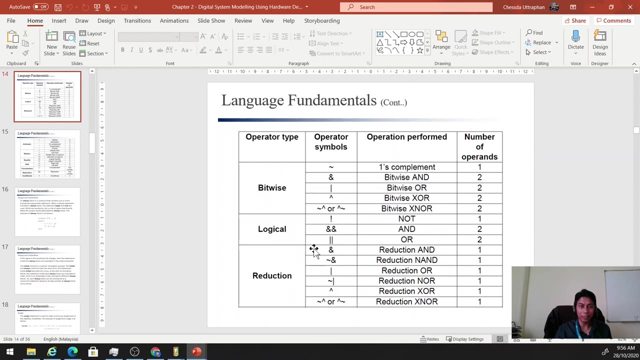 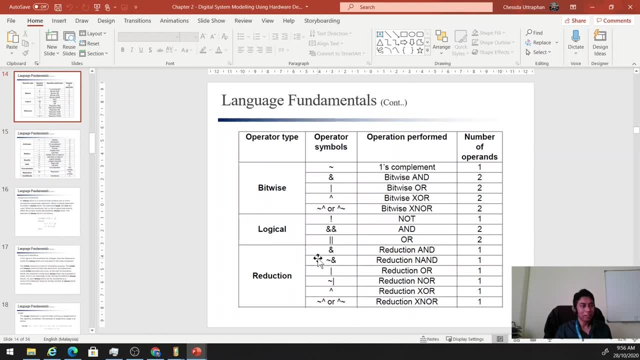 so remember. we are an engineer. we always so remember. we are an engineer. we always refer to the manual again, refer to the manual again, refer to the manual again. don't, don't, don't, don't memorize the menu, don't memorize the menu, don't memorize the menu right. 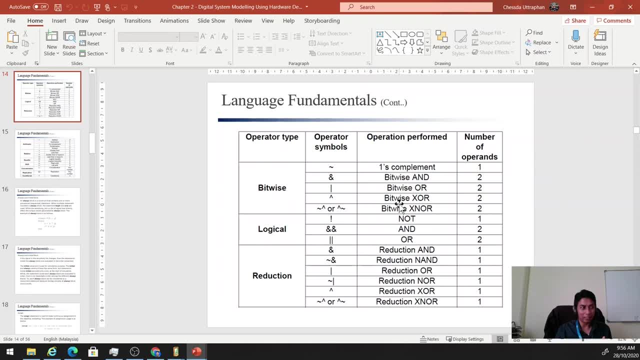 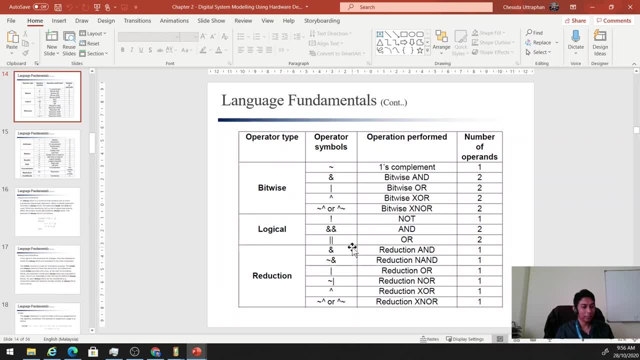 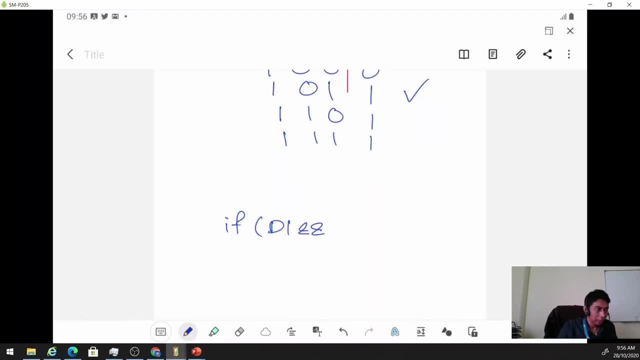 yeah so, yeah so, and logical and and logical and and logical, and when we want to test, when we want to test, when we want to test something, we use logical, and so they something we use logical, and so they something we use logical, and so they double, double n. 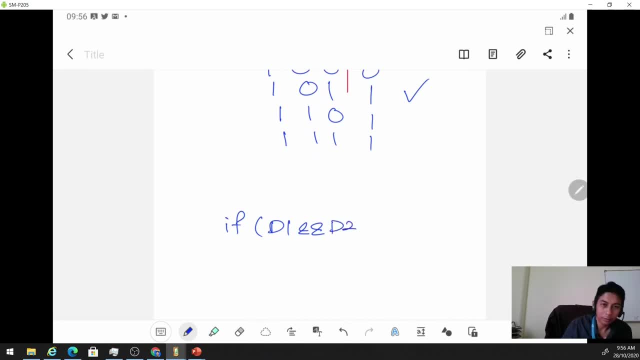 if d1 and if d1, and if d1 and d2, d2, d2, can, can, can, maksudnya kalau d1 1 and d2 1, maksudnya kalau d1 1 and d2 1, maksudnya kalau d1 1 and d2 1 alarm. 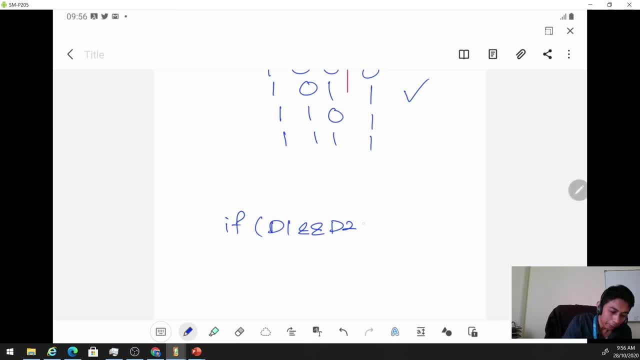 alarm. alarm activated right. activated right. activated right. or, or, or can, can. can you believe that? oh, you believe that, you believe that. oh, you believe that you believe that. oh, you believe that. okay, okay, okay, oh, oh, oh, d1, oh, d1, oh, d2, oh, d2. 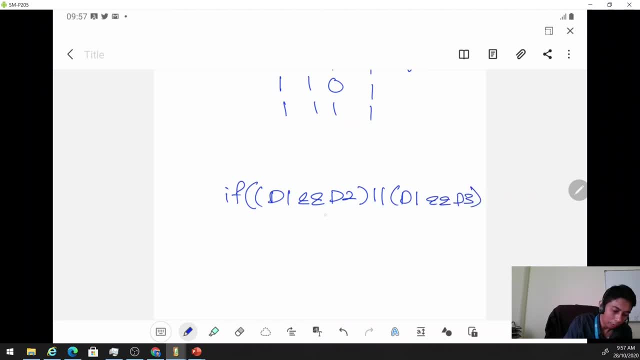 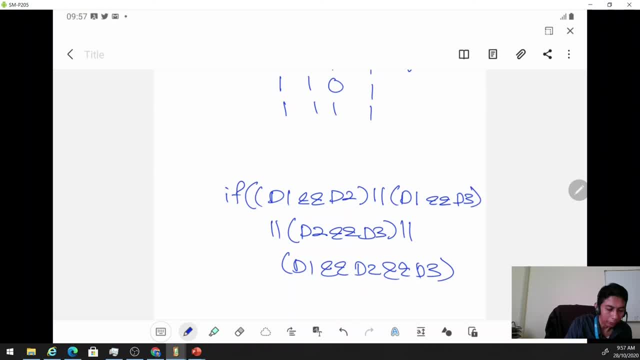 you can eliminate this one because it include it's not include all of it. so if this equal to 1, or if this equal to 1, or if this equal to 1 or 2, if this equal to D2, D3 through a equal to one l means that other than this l. 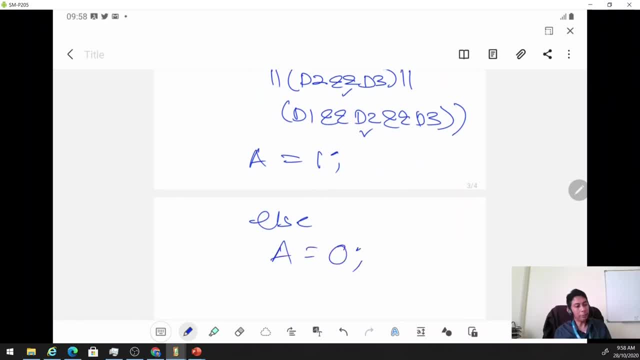 a should be equal to zero. so this is the bin area. all right, you get an idea. uh, all right. uh, i repeat, yeah. so this is the behavior we ask. we ask if d1 and d2 true, true, equal to one, all right, true if the condition is made true: d1 equal to one, b2 equal to one, yes, 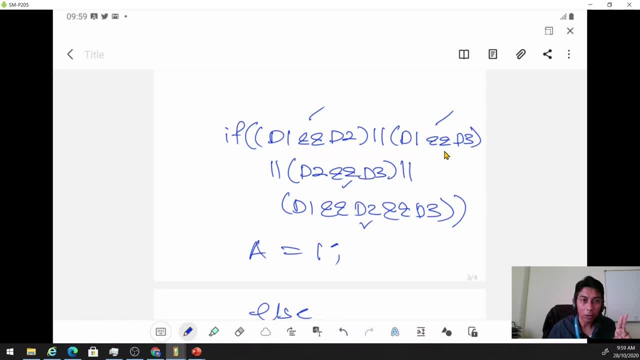 or d1 and d3 are open, all right, or d2 or d3 or all of the door are open, then a should be one. alarm is activated. else, other than this combination, a should be equal to zero, all right. so this is behavior, okay, meaning that this application you can. 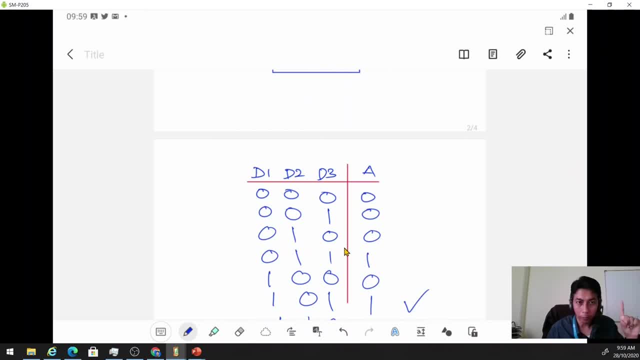 you can model using, of course. number one is data flow, because you have the boolean equation. now, from the tool table you can derive the boolean equation and you can do the behavioral modeling. and the last one, you can do the, the structural modeling, because from the uh, from this and from the, the boolean equation, you can derive the. 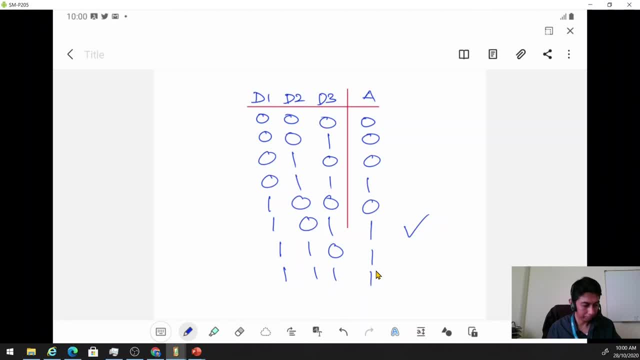 boolean equation. from the boolean equation you can derive the boolean equation. okay, alright, so so all right, so pakai mana-mana satu. Alright, In this case, mana-mana satu. jelah yang menggabung. Kalau you dah pakai data flow, pakai. 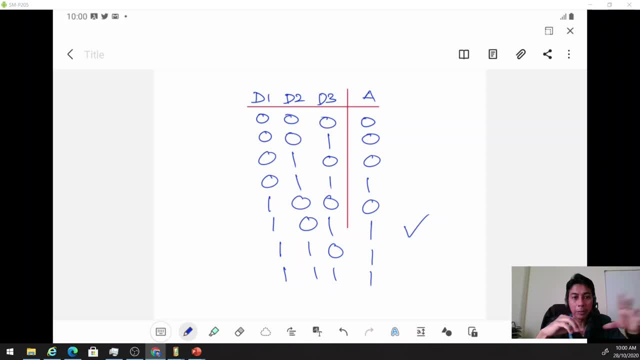 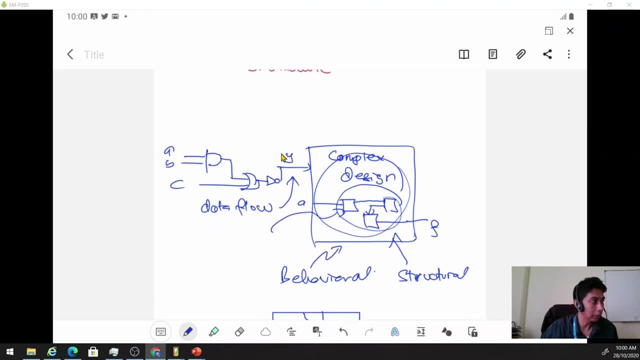 data flow jelah Sometimes. sometimes, macam this example, kan the circuit is complex? Alright, Sometimes, here, this part you may need to use data flow, Tapi this part you may need to use structural ataupun behavioral. Alright, And you.